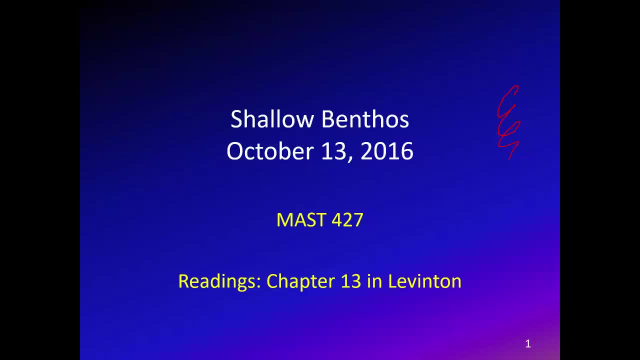 Okay, today we're going to be talking about another benthic environment, that's in fairly shallow waters, although deeper than what we saw for the rocky shore and intertidal pools. So for most of today's lecture I took it from chapter 13 in the Leviton textbook. 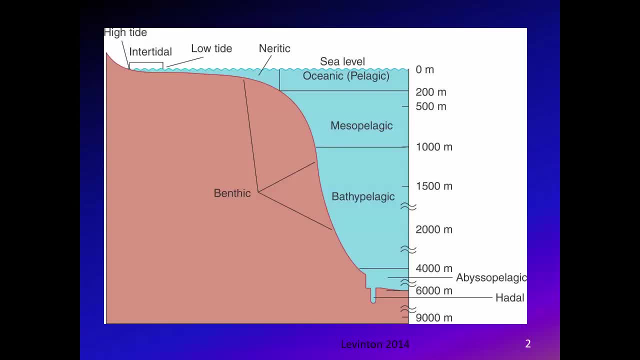 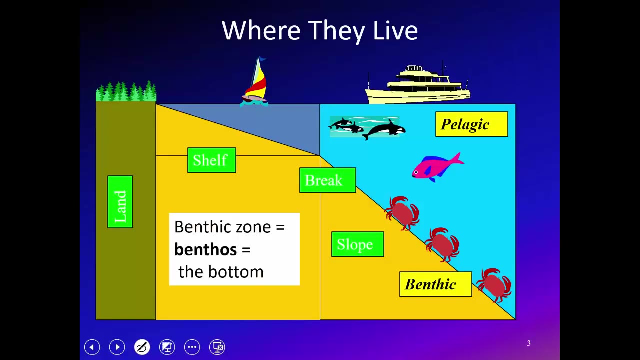 So, yes, as I said, we're moving up the benthic environment to much shallower waters, probably about less than 50 meters, 100 meters or so, but not quite as shallow as the intertidal pools that we talked about already on Tuesday. So here's just another diagram showing that. 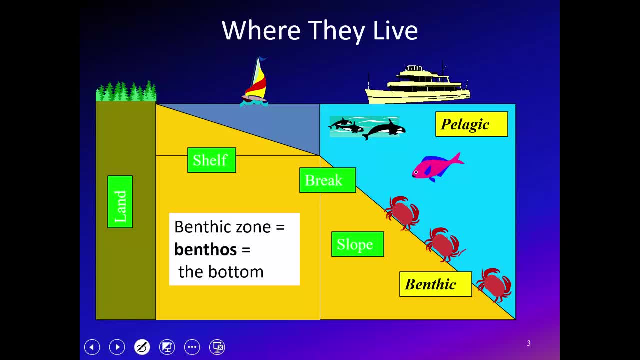 gradient in benthic environments, ranging from the deepest ocean, of course, and to the shelf, And for the most part we're talking about environments that we see on the shelf in shallower waters. I'll go back and forth between talking about benthic zones. 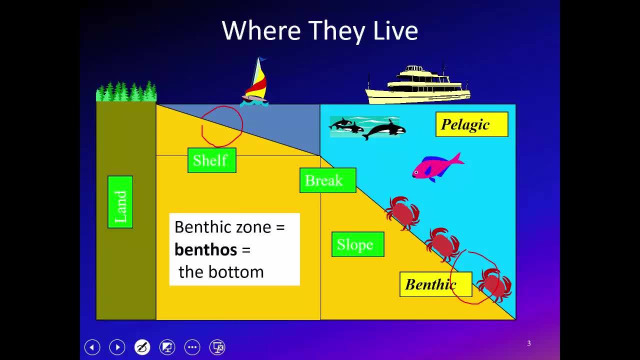 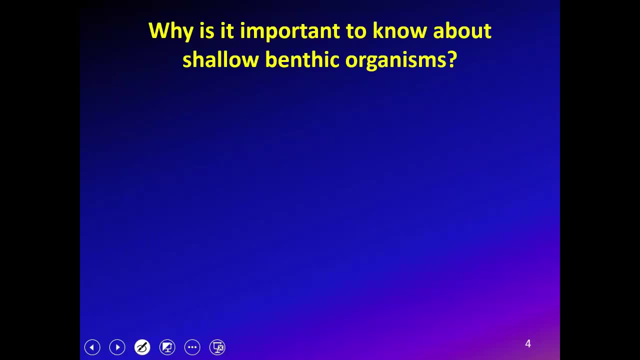 and the benthos, Benthos, of course, being the noun meaning the same thing as benthic zone. So why should we know about these, these organisms and this environment? Lots of reasons. One is: if you didn't care about invertebrates themselves, we're going to be focusing mainly on invertebrates. 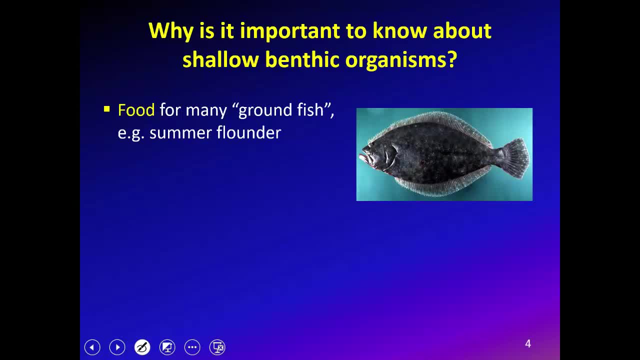 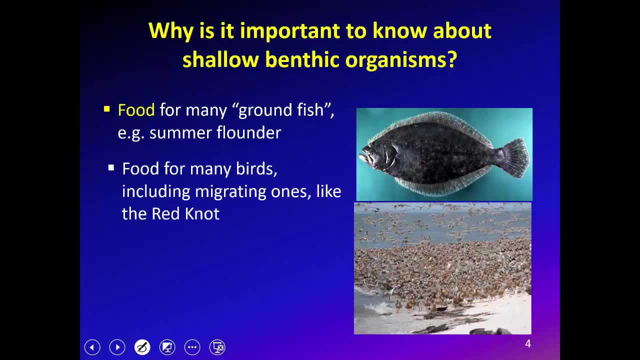 today. They are food for organisms that you may care about, that is, fish, in particular ground fish that feed off of the on these organisms. They're also food for birds such as the red knot, which is a migrating bird that we see very common here in the Delaware. 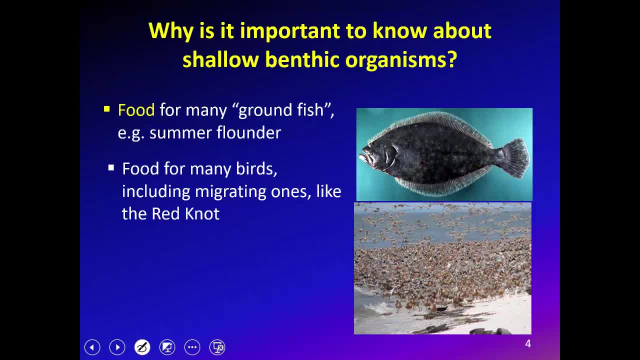 estuary, And when we talk about estuaries I'll get more into that topic, about the importance of our estuary in supporting these migrating birds. These shallow environments are also important biogeochemical cycles- just to say a few words about that in a minute, And then, as always, 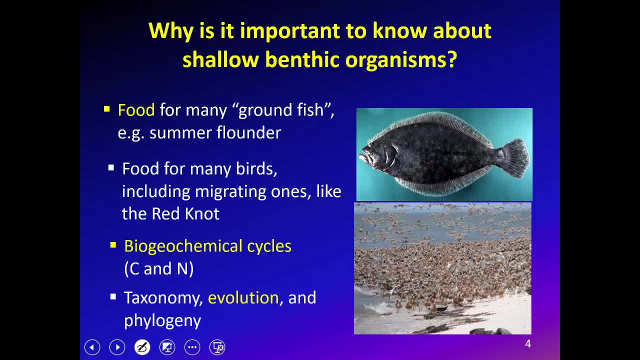 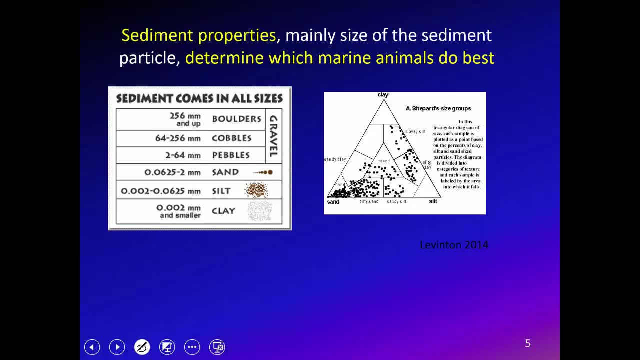 in general about the evolution of organisms, we need to look at marine ones, and that includes many of those that live in shallow benthic environments. So in talking about these, these environments, it's important to look at the sediment and the qualities of that sediment. It 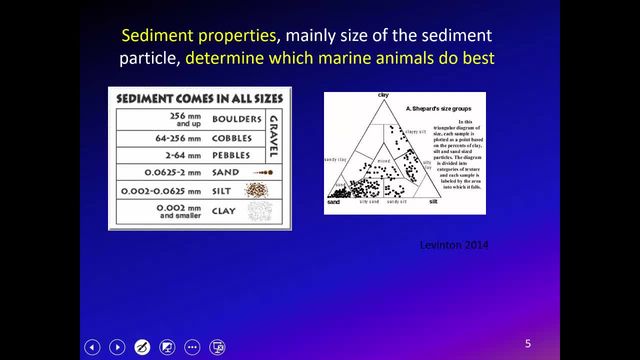 varies quite a bit, from very coarse material- not quite boulders, but certainly coarser material- to very small particles. And that has a big impact on what organisms are present And basically the sediment characteristics depend on the currents. So basically, if you have very 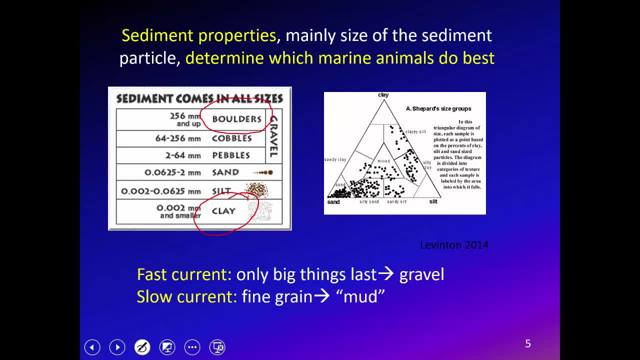 strong, fast currents. only big things are going to be able to stay in that benthic environment, that place That would be more like gravel, of course. And then the other stream is very slow currents, weak currents. And then the other stream is very slow currents, weak currents. 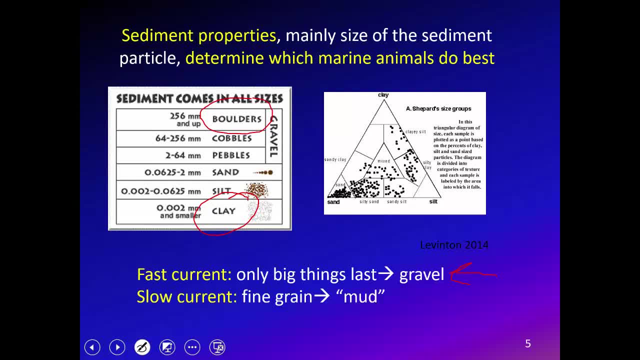 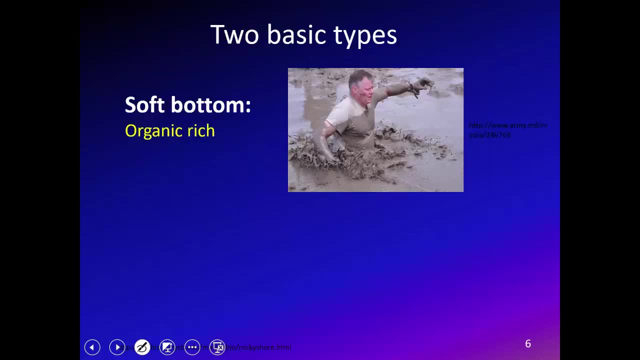 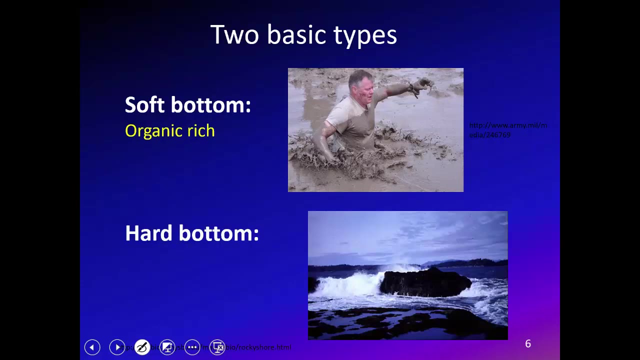 many other things can settle down and build up in that place, So it'd be more like mud And also turns out to be more organic, rich than what we see with gravel, And so we can divide these sediments into two basic types- really technical here, soft and hard. 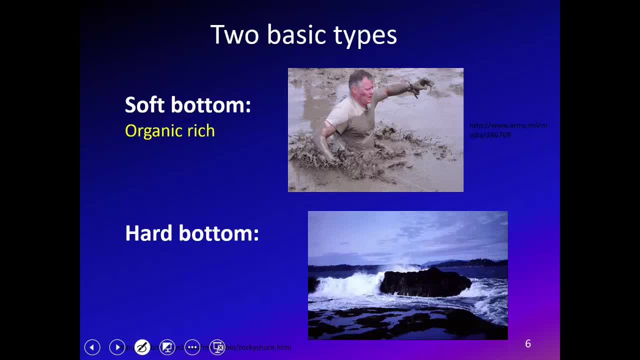 bottoms And for the most part today we're going to be talking about soft bottoms, And these places are, for the most part, rather organic, rich, as kind of implied by this poor guy going through this mud bath. I think it's some training exercise or some race that involve going through mud. 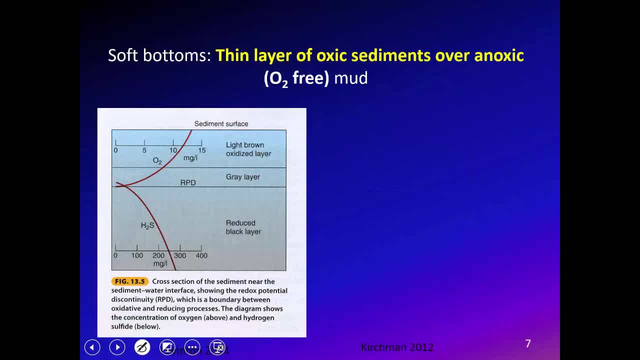 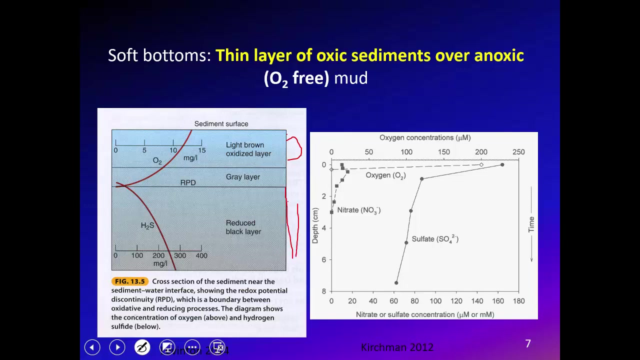 Anyway, what's really characteristic of these soft bottoms is the fact that they are basically a very simply two zones. One, a very thin layer of oxic sediments, that is, oxygen rich sediments, above a much deeper layer of potentially very oxygen poor. 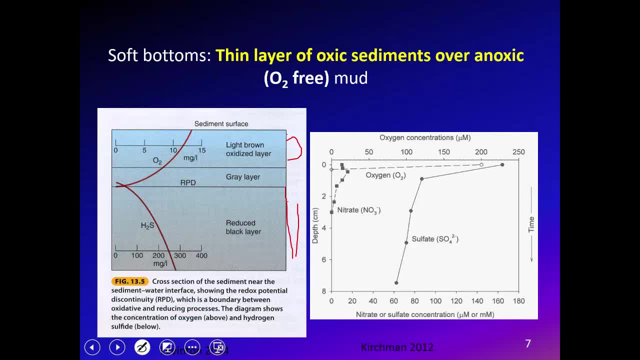 even no oxygen, that is anoxic sediments underneath that thin layer. So the graph on the left kind of illustrates that a little bit, shows the buildup of hydrogen sulfide, which is a poison for most organisms. That's the result of sulfate reduction. 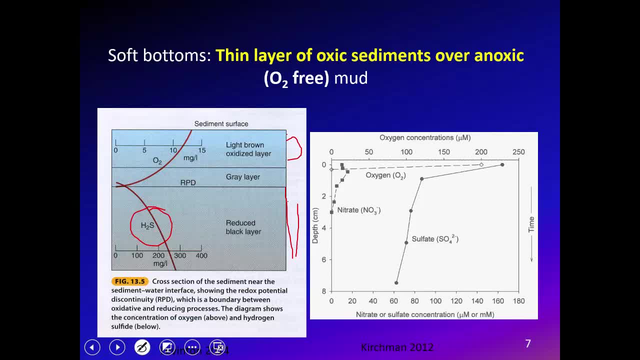 the type of metabolism that bacteria carry out and they produce hydrogen sulfide And that hydrogen sulfide can be really high and deep down in the sediment core but then, as it reaches near the surface, it goes down to zero. Oxygen does the opposite. 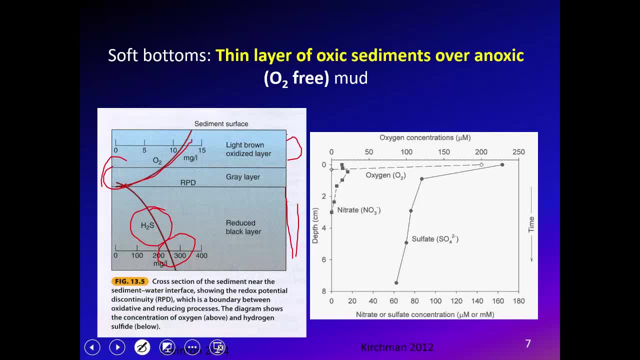 goes from very high concentrations in the surface to very low concentration, sometimes quite quickly, in the sediment profile. So that's illustrated. perhaps I think a little bit more clearly Again on the right here so you can see again oxygen disappearing. You can see within. 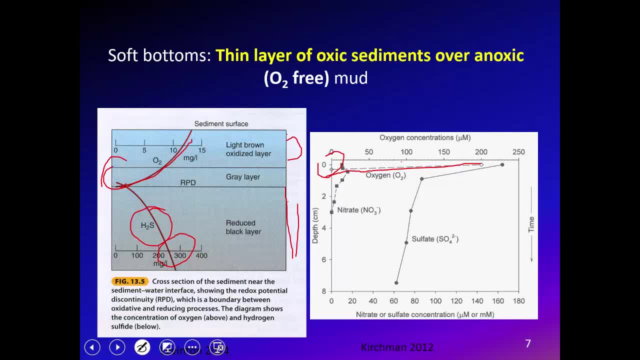 just millimeters, less than a centimeter, less than a few inches, much less than an inch. there's no oxygen at all and you see the decrease in sulfate, and what's happening here is that the sulfate is being reduced down to hydrogen sulfide, and hydrogen sulfide as 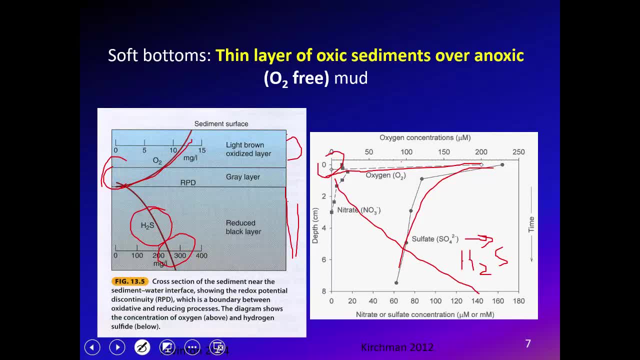 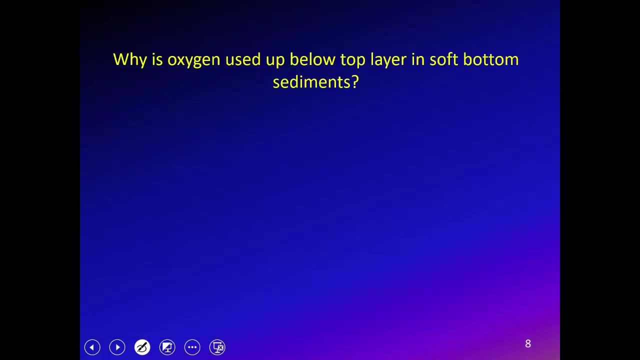 I mentioned is a poison that a lot of organisms have a lot of problems dealing with. Sulfate Reduction僕 x 2 x 3, that's one. main characteristic of these soft bottom sediments is this two-layered system: oxic sediments on top and anoxic sediments underneath. so why is oxygen used up in the 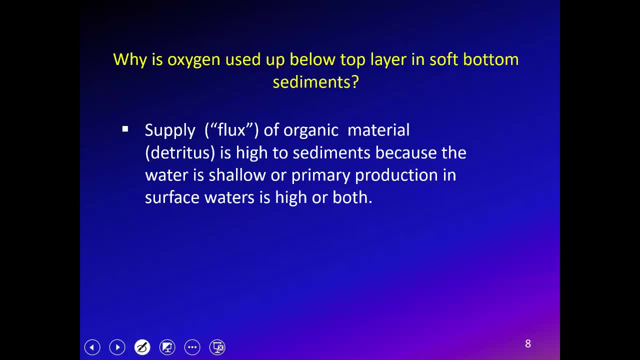 top layer, for one thing is that these environments see a lot of organic material, so the flux or the supply of the organic material, mainly in the form of detritus is is quite high, and so that's that's um. that's the case when the water's shallow less than 50 meters and also you have to have high. 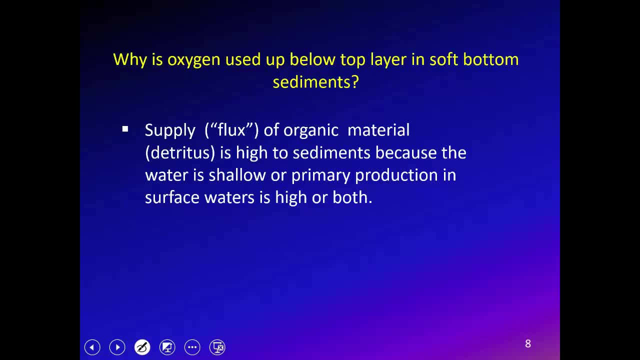 rates of prime production and generally, often during close to a coast, in shallow waters like this, you can you can see high prime production, so you need to have both now. the other part of the equation of the equation is: is that the diffusion of oxygen into these sediments? 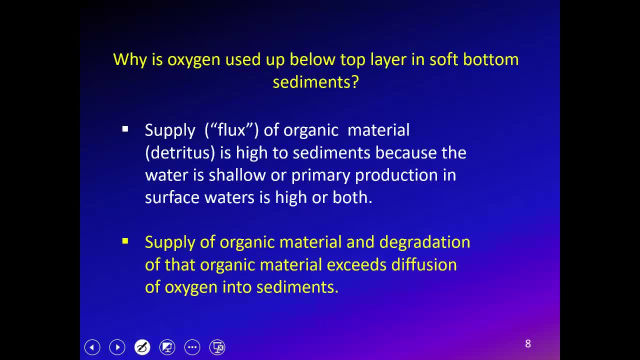 is just not enough to keep up with the supply of their organic material. so there's more organic material going into these sediments than there's going to be in these sediments. so there's more organic material going into these sediments, so there's more organic material going into these. 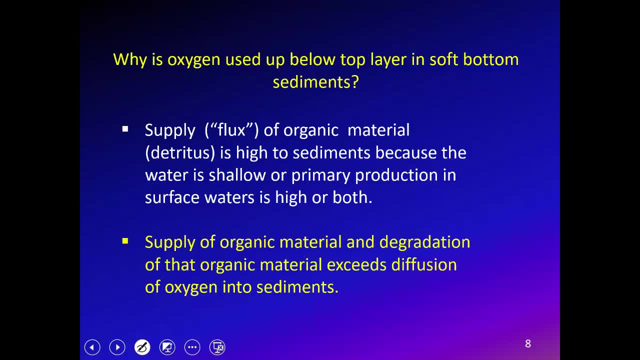 sediments. so there's more organic material going into these sediments, into that, into that sediments, and that organic material is degraded by the bacteria, mineralized by the bacteria for the most part, and that uses up all the oxygen. it uses up the oxygen faster than the fusion. 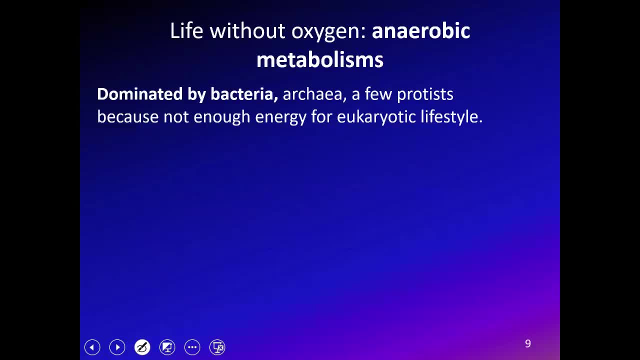 can replace it. so that's why you get to the uh, the uh, the uh. the lack of oxygen, um below a few millimeters um in the sediment core. so when you don't have oxygen, basically it you're the uh the. the life there is dominated by small organisms. 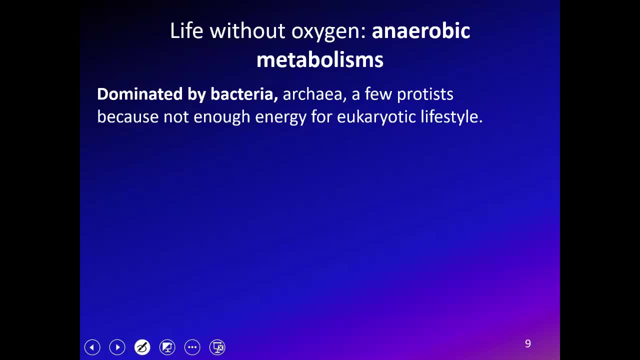 mainly bacteria, archaea. there's a few single cell, eukaryotes, protease, that are able to survive there. later, when we talk about dead zones, which is a problem that we see in coastal waters, we'll see that there are some um larger organisms- metazoans- that are are able to withstand the lack. 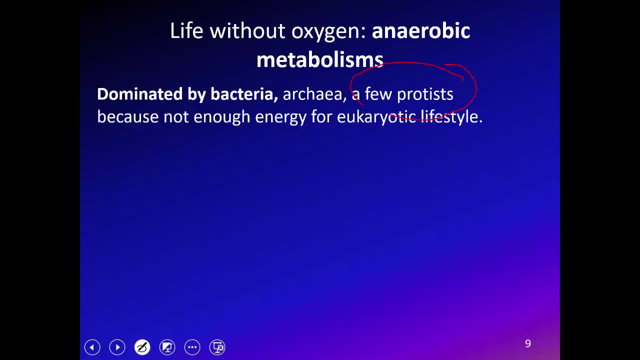 of oxygen for a limited amount of times, a little amount of time, but that's, for the most part, the exception rather than the rule. for the most part, only organisms that are very small- bacteria and archaea, and a few produce- are able to survive without oxygen. so the types of anaerobic 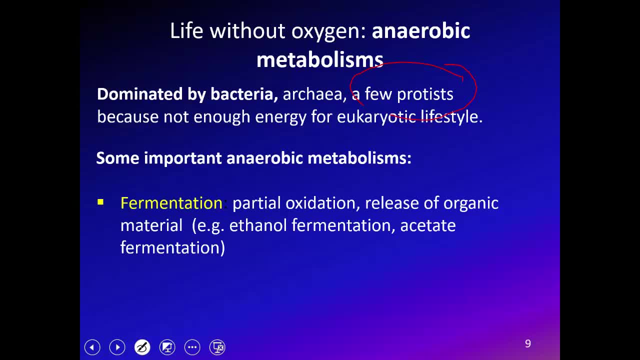 metabolisms, that is, metabolisms without oxygen, include fermentation and that you actually enjoy. if you, for example, i have yogurt with my cereal, so that's a yogurt is a product of a fermentation. ethanol- not with my cereal necessarily most days- is a fermentation byproduct and there are many other ones. i mentioned already sulfate reduction: sulfur reduction is carried out. 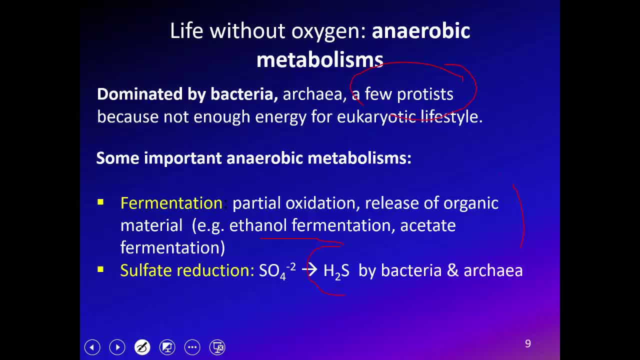 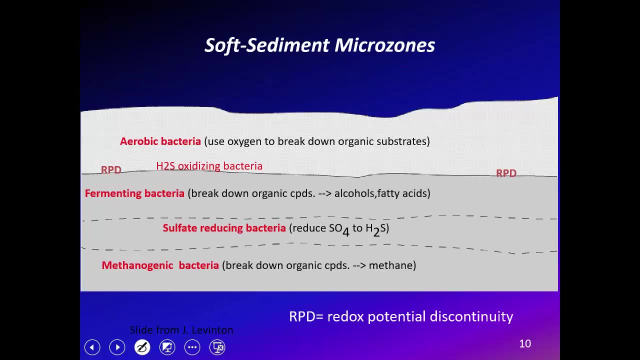 only by bacteria and archaea, and it produces this toxic gas that's toxic to many higher organisms, um. and then, finally, methanogenesis is the? uh, the synthesis of methane. um, that's done only by archaea. so here's another diagram showing the, the layering of these, these uh um organisms, uh, and. 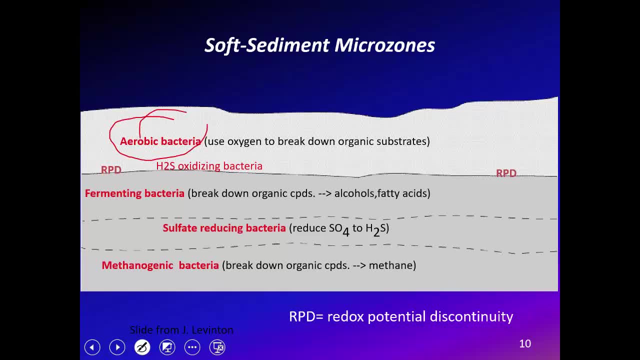 at top we have the aerobic bacteria and other organisms that use oxygen. then we have the fermenting bacteria, finally the sulfate reducers and then the methanogenic. but that's the maximum mistake. the textbook- l follemton's uh textbook- has bacteria, those that's only done by archaea and that's seen only down deep in the 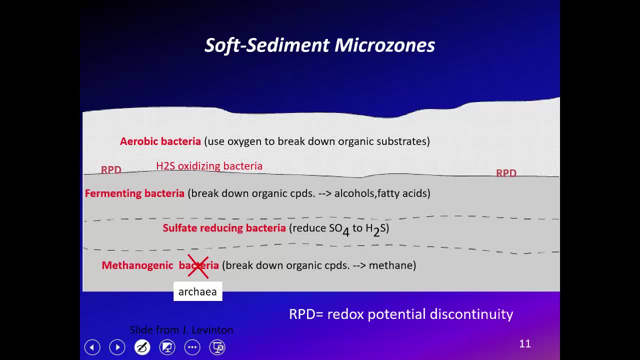 assignments. so, uh, again we see this two layered system with oxygen, a lot of oxygen here, and and oxygen below that oxic layer there's no oxygen at all. so that's sometimes called the redox potential discontinuity. at least that's what levin calls it. i really don't use that term. that that important. 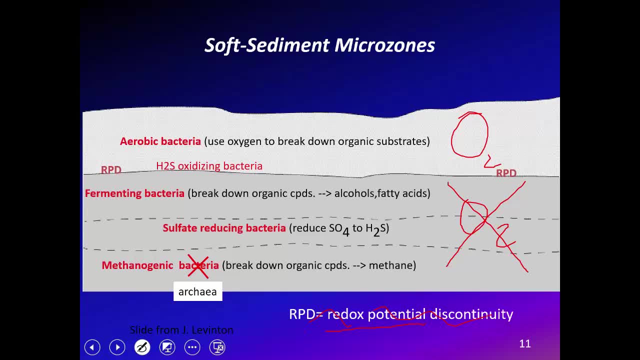 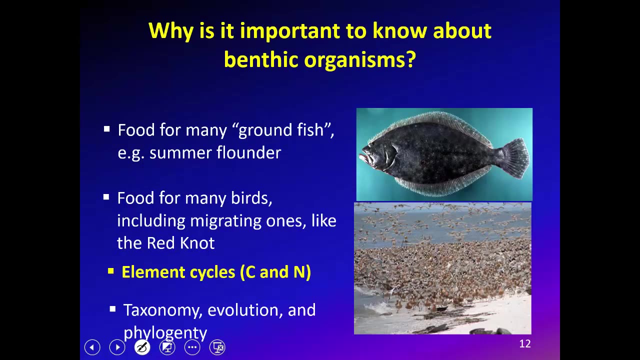 for you to remember. what is important for you to know is that there's in these sediment habitats, the only a top layer of those sediments has lots of oxygen. the rest does not. now, the exception to that is is what benthic organisms can do to those sentiments. 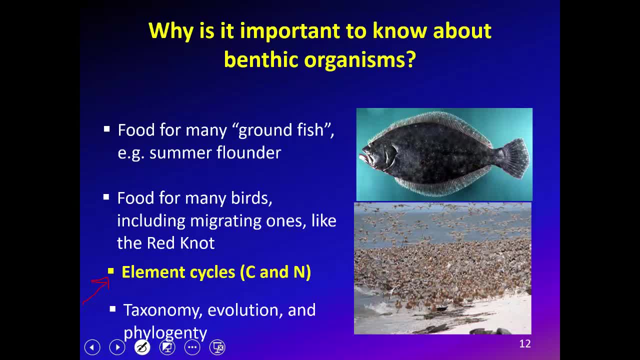 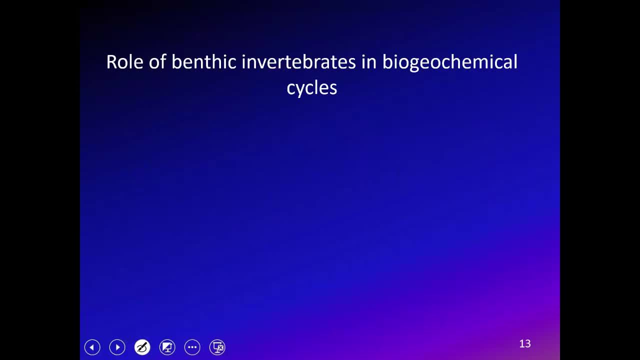 and that plays into the importance of these, these organisms, in terms of element cycles and so really in terms of biogeochemistry. in the carbon cycle in particular, the role of benthic organisms is basically the breakup to the detritus, and we'll talk quite a bit about detritus and i'll give a bit more. 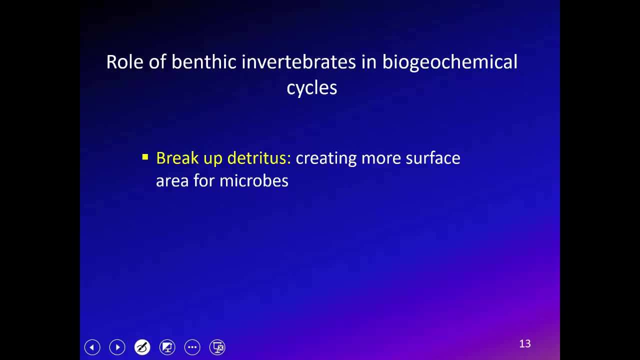 precise definition of what that is in a minute, but suffice to say for now it's a it's non-living organic material. so what these benthic invertebrates do is that they break it up, and that carries breaks, creates more surface area for microbes to do the hard work in terms of 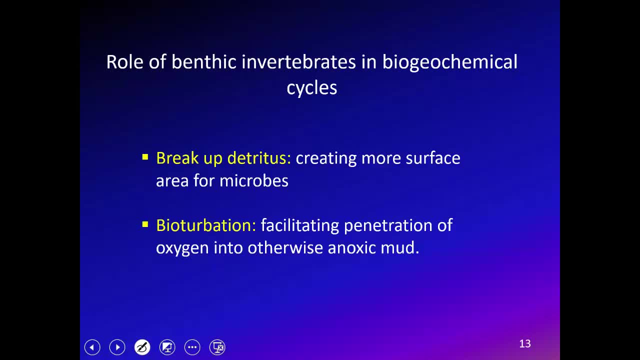 mineralize it back to the inorganic constituents like co2, ammonium and phosphate. the other main role of these benthic invertebrates is to mix up the, the sediments and and the word that's used to describe that that mixing up is bioturbation. 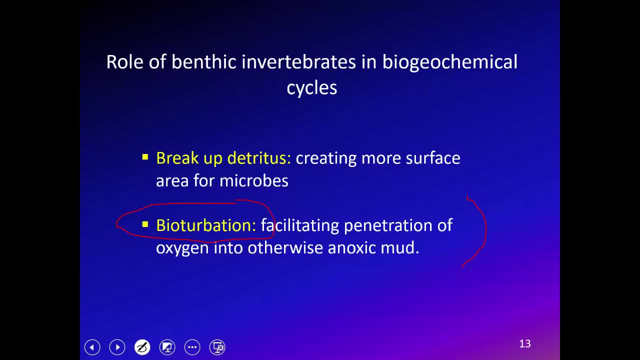 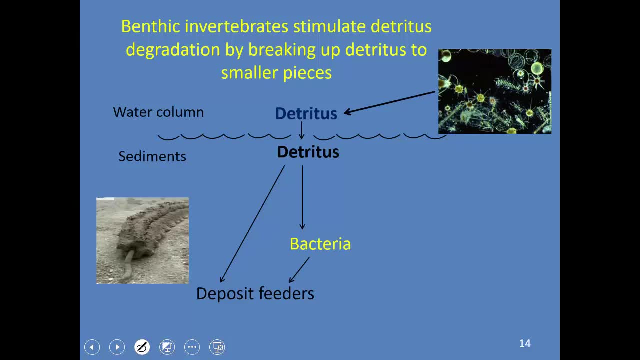 and basically that allows oxygen to get down to what otherwise would be just oxygen-free or anoxic mud, excuse me. so, so what? what the invertebrates are doing basically is that they're feeding on this detritus, this non-living organic material, and, uh, we'll, we'll see later in class i'll show the show you the picture or video of what this. 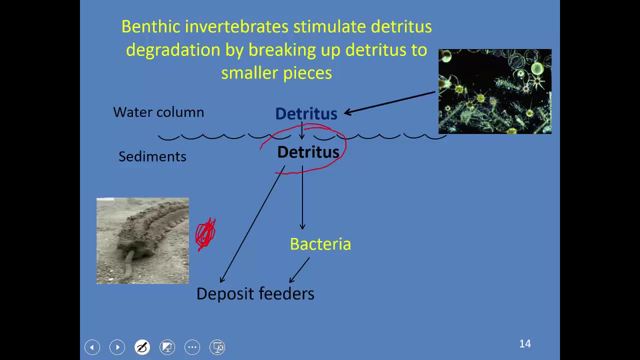 sea cucumber is doing there, like maybe you can get an idea what it is doing, but anyway, we'll get into that a bit more. but suffice to say that these deposit feeders- and we'll see in a bit, uh, in a bit what those are- are eating the detritus and and they are also 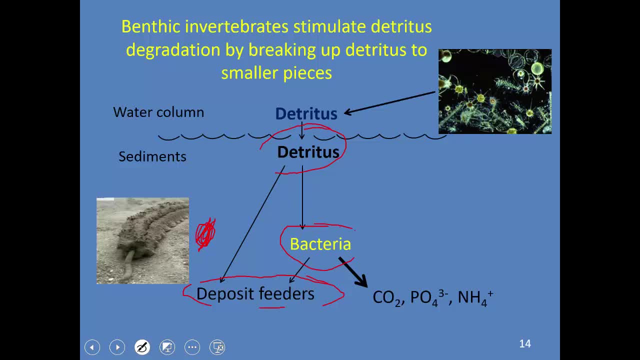 eating the bacteria and in the process of doing that, the bacteria then release the inorganic constituents of that detritus, turning that organic material back into its inorganic constituents- co2, phosphate and ammonium- and of course that can be then released back up into the water column and fueling prime production that we see. 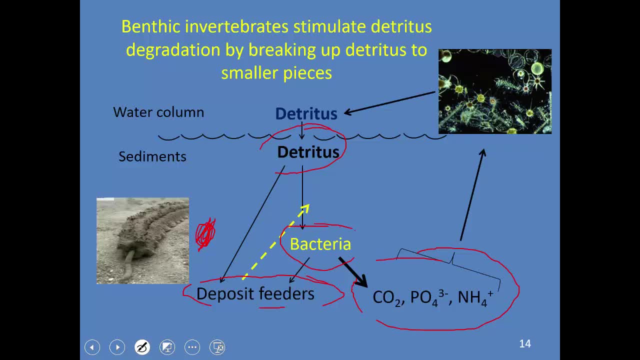 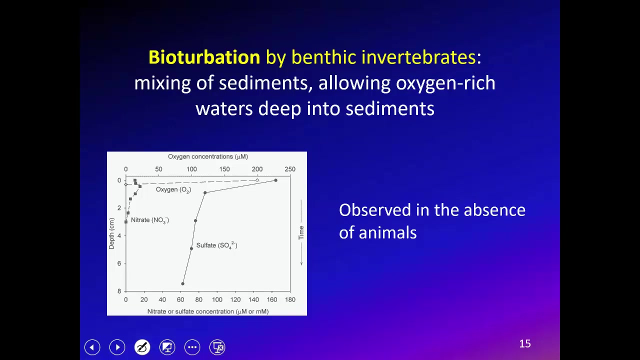 in the water column. what the deposit feeders are doing basically is they're making smaller bits of detritus and creating more surface area for bacteria to do their job. now, the other role of these benthic invertebrates, as i mentioned, is to stir things up to bioturbation to carry out. 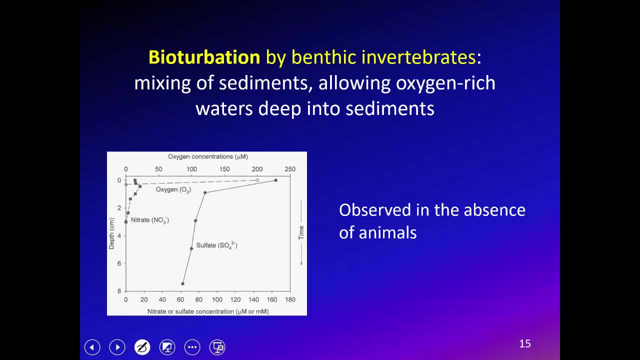 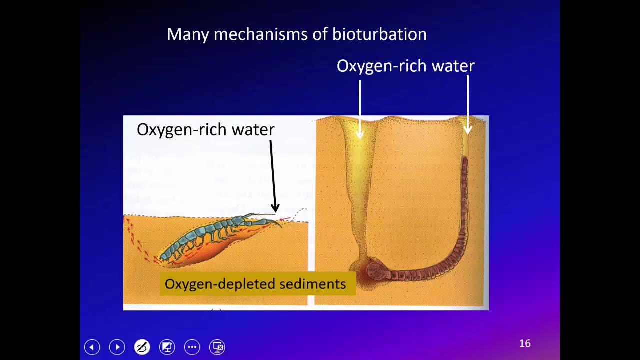 bioturbation and basically this nice pretty picture of oxygen disappearing within millimeters and the sulfate disappearing like that and nitrate also disappearing. you really only see that when you don't have any animals mucking things up. so what the animals do is basically they. they do this as 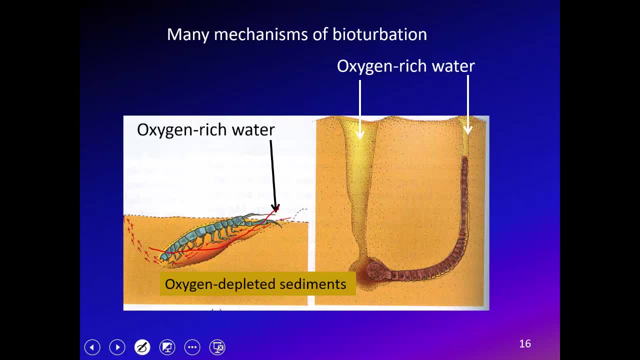 i mentioned bioturbation. they basically bury a barrel into the sediments and create little channels and mix things up, allowing oxygen to oxygen rich water to get into the mud that otherwise will not be able to get there. that's a much faster way to get oxygen down into sediments than than simple diffusion. 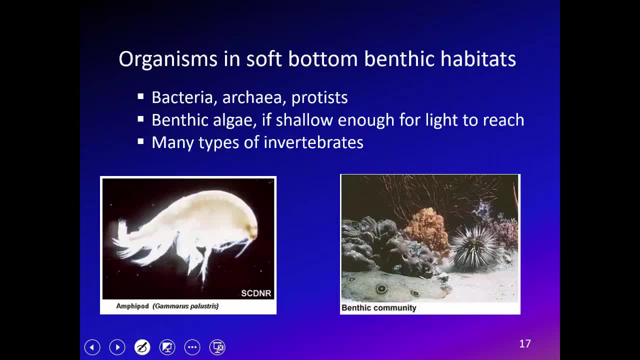 so that's one reason why to have these oranges around in these benthic environments is to put more oxygen into the sediments, which helps all organisms and helps actually degradation of that material. and then also they break up the detritus to make smaller particles. 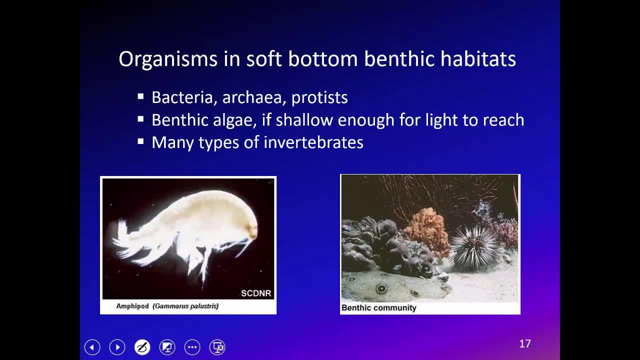 and then they're able to get into the mud and create more surface area for bacteria to do its work. so let's now look at some of these organisms that we see in these, these habitats, and basically there aren't any new ones. there are a few new ones perhaps, but you've seen many of the names already. 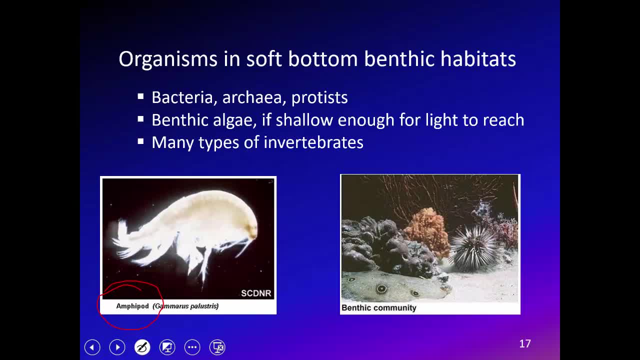 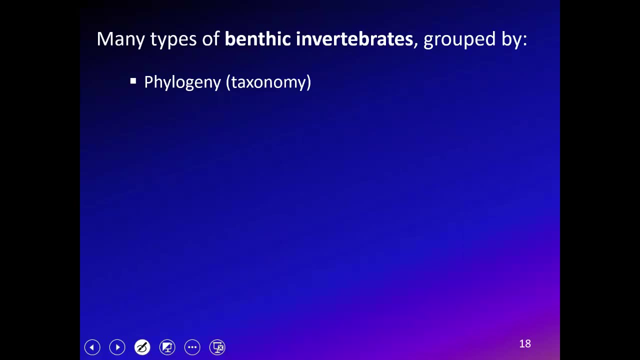 here's an amphipod. that's one of the words, genus names or or types of organisms that i want you to remember. but we'll get into a few other ones, but i don't think you'll. there'll be any surprises. we've seen already for starting with the zooplankton and then other invertebrates down in. 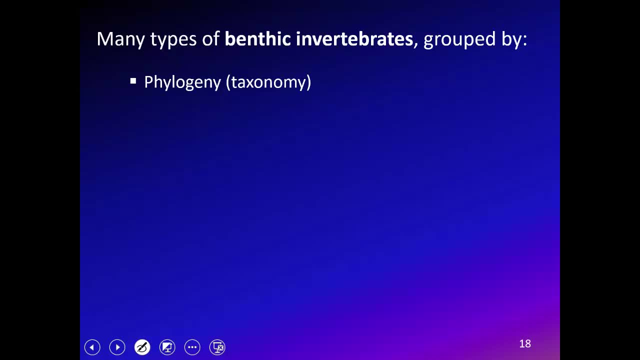 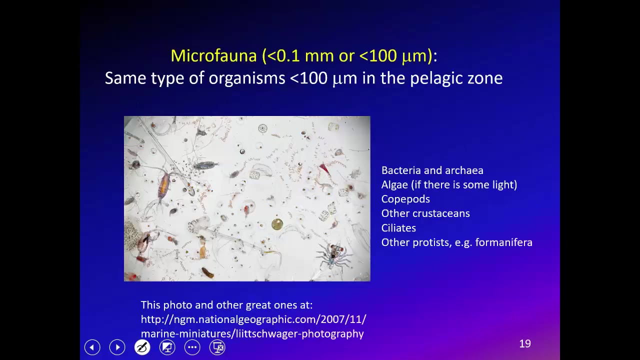 the deep benthos. we can divide up these shallow, uh benthic invertebrates by phylogeny. that is just their taxonomic name. and of course we can divide them up by size, and we'll see in a moment. we can divide them up by other ways, which we'll get to in a minute. so size let's. i think in the past i've 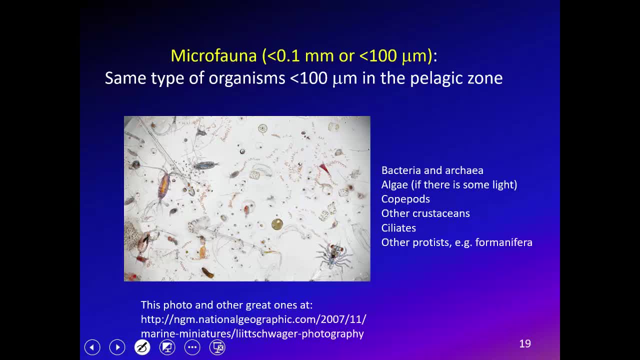 started with the biggest and going down to the smallest. let's start with the smallest and go to biggest. microphonic includes all sorts of small organisms that you've all seen before the. you know i put bacteria and archaea here, but but you know they aren't really fauna at all, but certainly these. 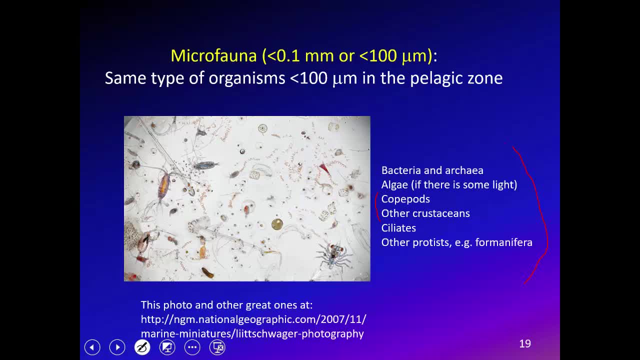 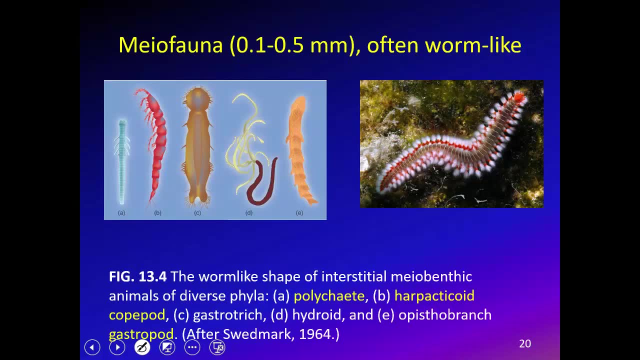 copepods, other crustaceans, ciliates and so on are important members of this microfauna- myofauna- again a word that you should know already. these are 0.1 to 0.5 millimeters in length. they have this characteristic of being worm-like, even though they're not really. 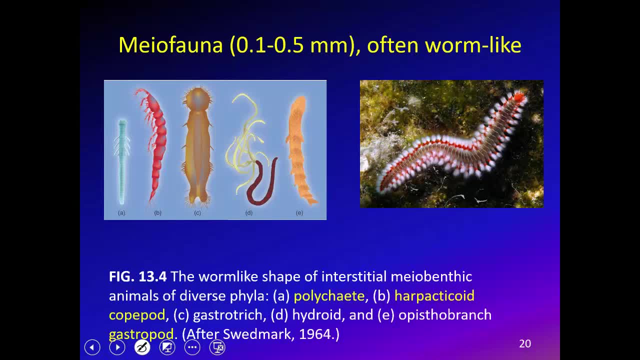 warm. they have a worm-like shade, including the polychaetes. that's a word that i want you to know. they're herpacticoid copepods, you know again. this one even looks less like in the copepods we saw in the water column, but that's, that's a herpacticoid copepods, or those. 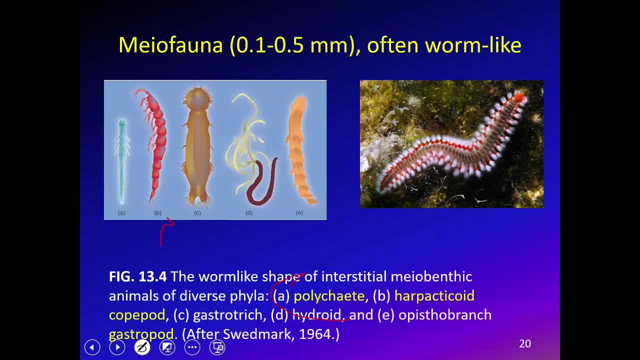 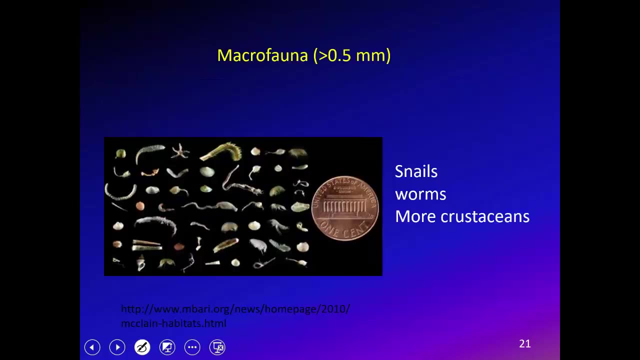 copepods that we see in the benthic environments, as opposed to the to the water column and so on. so these organisms have in common is that they have this worm-like shape, which helps them kind of get in between the cracks of of the mud and clays that we see in this environment. macrofauna, of course. 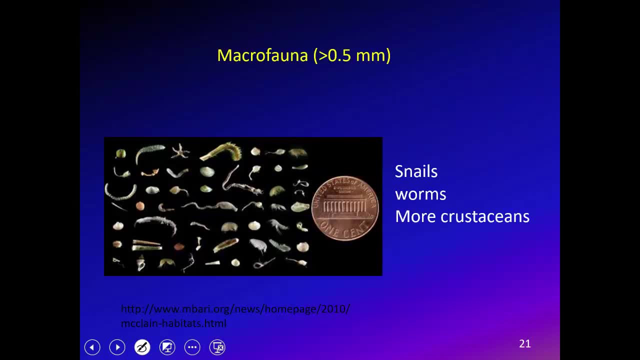 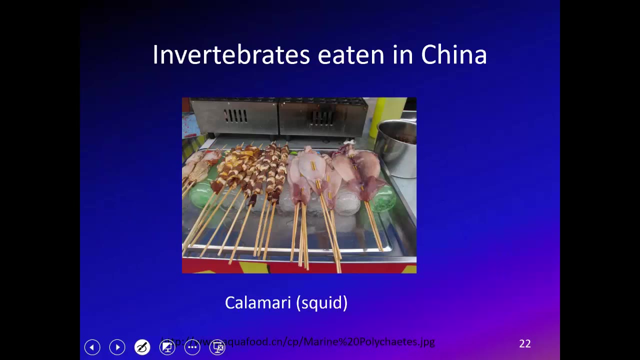 these are bigger organisms. rather than giving you a list of the of organisms that i want you to remember, i thought we'll just take a little break and i'd like to show you a few pictures from a trip i went on last spring to china, saw lots of my wife and i saw lots of things that were eaten there on the street. most of these: 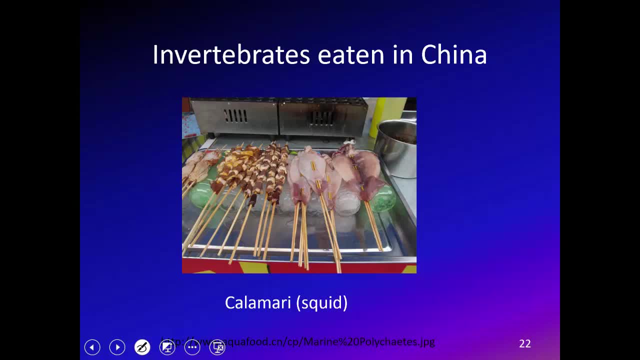 pictures i think are from beijing, some of them are also from qingdao, qingdao and xiamen. xiamen- we went through all three of those places, but xiamen is is a city located on the coast of china and it's the university there has a cooperative agreement with the university of delaware, which is 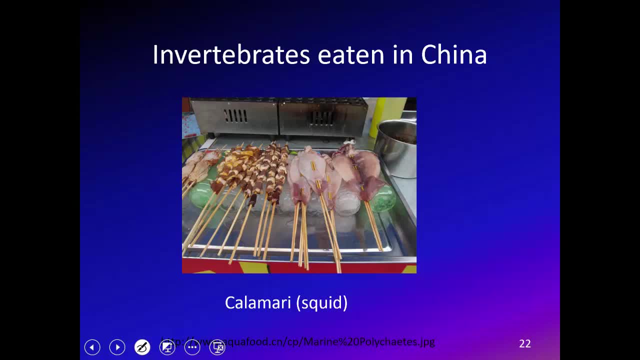 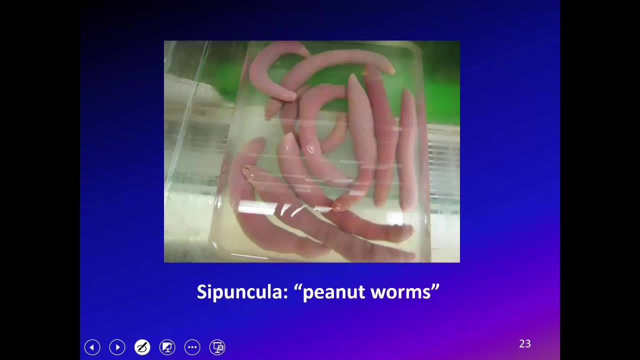 the reason why i went to xiamen. so anyway, um, you, probably even i have eaten- come up, uh, calamari- that's of course the italian word for for squid, but a little bit more exotic, that maybe you haven't eaten, that i didn't eat spinoculars, or they're peanut worms. 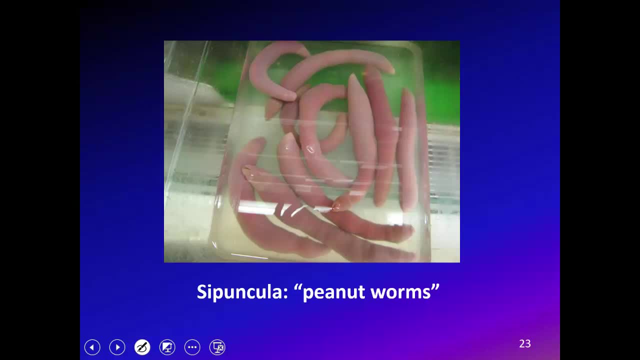 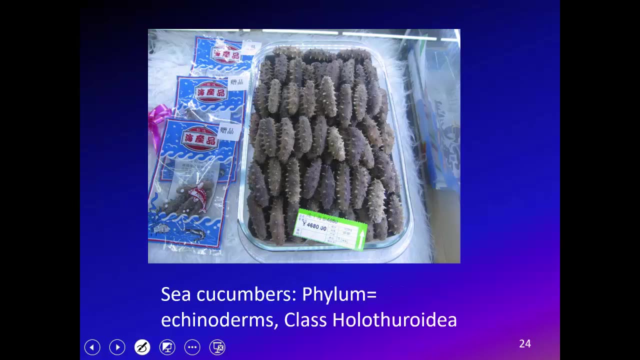 they are are. some folks put them in an analid phylum but others put them into their own phyla. and then you have the sea cucumbers. i mentioned about having those. i've didn't have them on this trip, but on another trip to hong kong i did have a sea cucumber, and 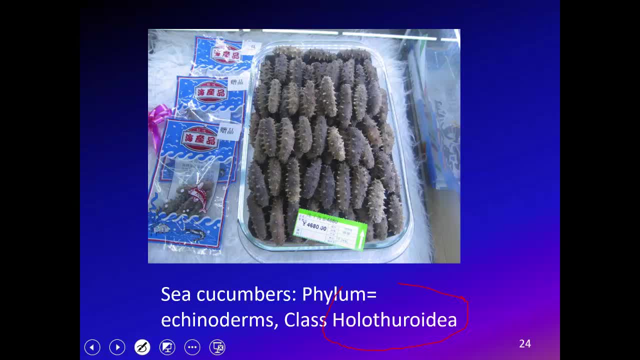 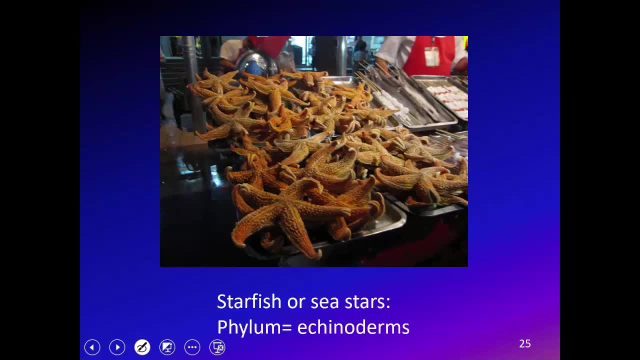 and i mentioned the fact that i'd like you to remember whole ethereans is there, there's a class that has the sea cucumbers, and then finally, and that's so, finally, i guess i one more picture starfish, or sea stars. um, these are echinoderms. um, that is a word that you should. 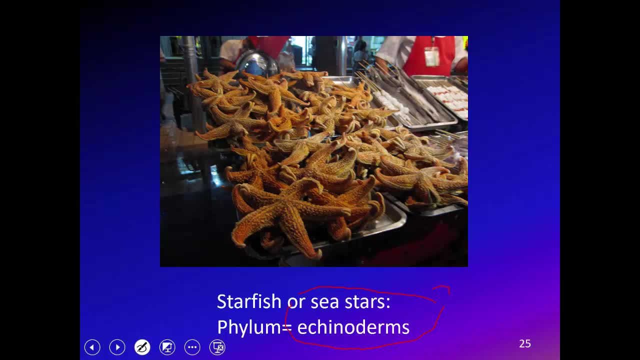 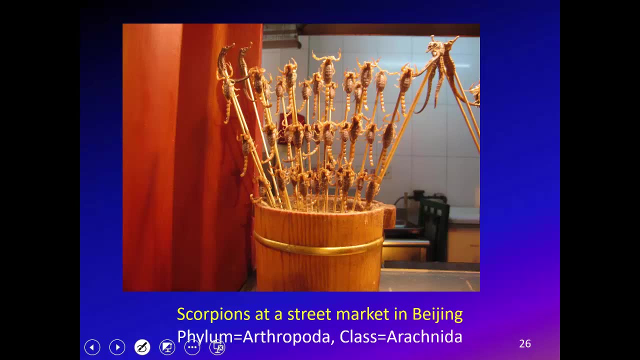 know, uh. and then this is the final picture- most bizarre, not very marine, but couldn't resist- showing scorpions. and what's not shown in this picture is the fact that these scorpions were still alive. they're still kind of wiggling around on those sticks there and i have to say i don't think i saw anyone actually. um, uh, buy them what? 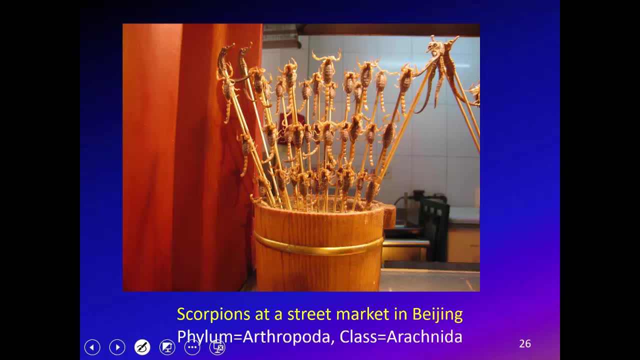 they would do is they would cook them up right there on the street and, like i don't know what, i suspect all you had was just kind of chunky, uh, crunchy, crunchy feeling, or whatever your mouth from, from the chitin exoskeleton. um i i didn't quite know when i was looking up the taxonomy of 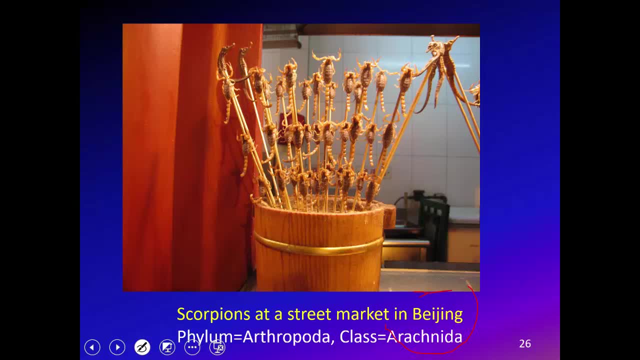 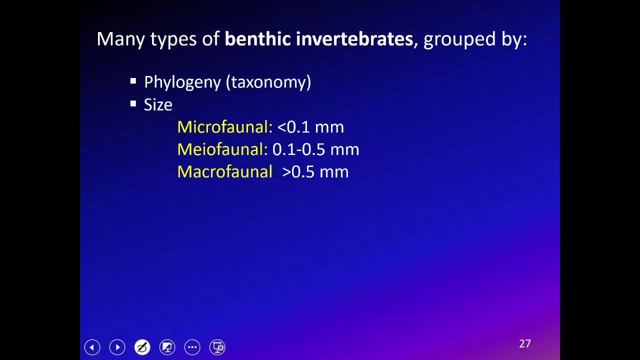 scorpions is that they are actually in the same class as spiders and arachnids anyway. so those are some of the organisms that that we, that that we see not, uh, not scorpions in chalabinthic environments, but some of the other ones that we see there. 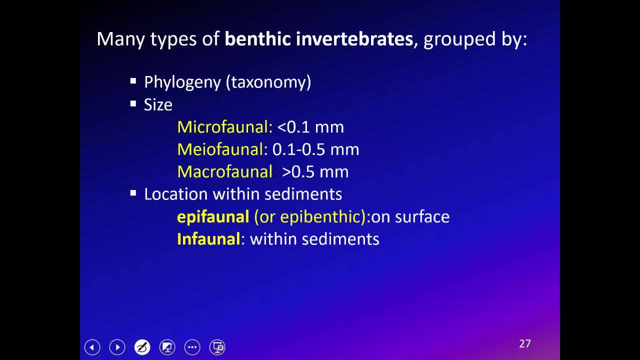 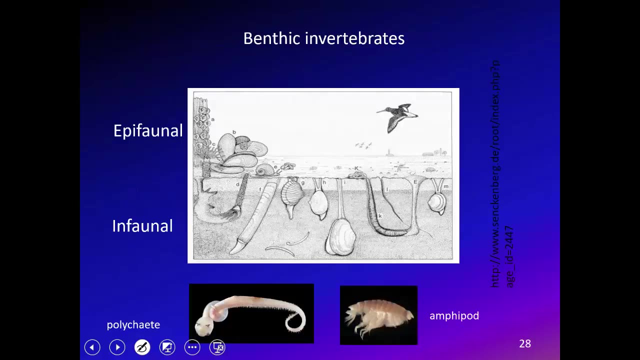 um. another way to divide up these, these invertebrates, is by where they live. um and uh. the two words there that you need to know are epiphaunal or epipentic, which means on the surface, or infaunal, which means in the sentiments and not that hard to to picture. basically a lot of. 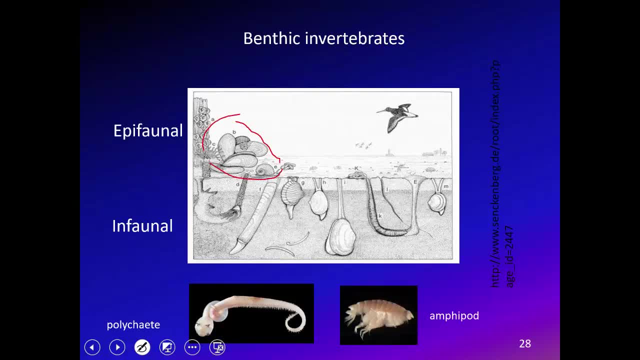 organisms are again just living on top of the surface. here's a gastropod, or his number of by vowels. and then, perhaps a bit more surprising, are these informal organisms that live within the sediments and the vengeance subside within them, so that that would be your way around the pandemic. 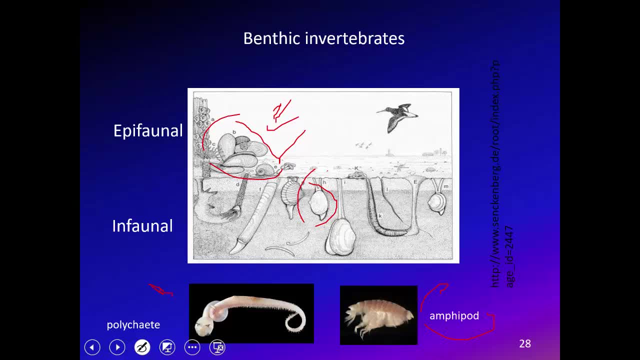 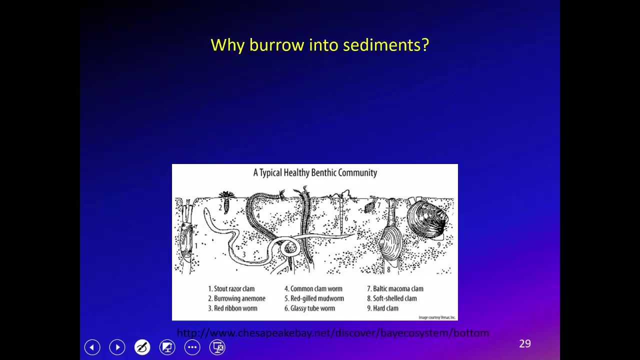 would include things like the polychaete here, or again the amphipod, you know, that shrimp-like crustacean that i asked you to remember, so, uh, so you know it kind of raises a question: why? why go down into the cements where you know there is a danger of encountering hydrogen sulfide, which 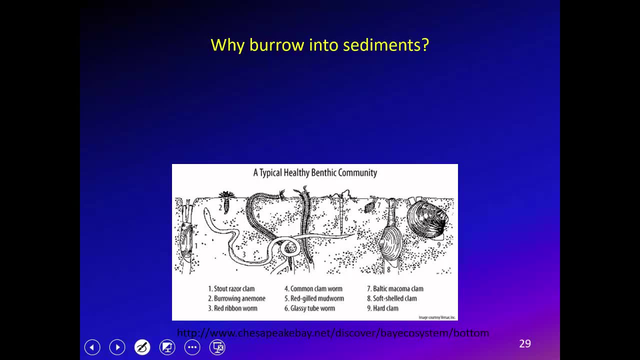 is a a poison, um, and why get down into the mud? and also, you know there's there's a chance of less oxygen down there. so why do that? why do you think they do it? well, there's probably two answers. one is that they probably get more food. they may go after some of the microbes that are. 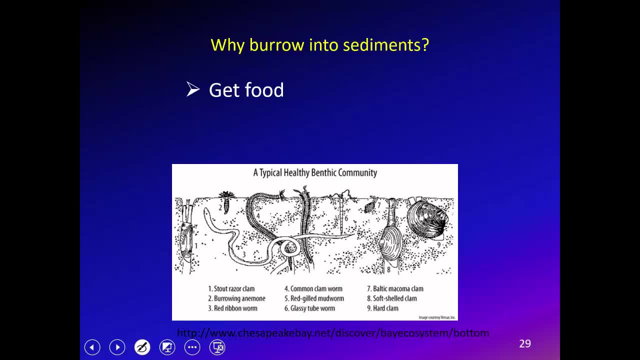 down there, other invertebrates perhaps to try this that's been buried there. and then another answer, i think, is to get away from organisms that don't burn, to get away from predators. you remember those fish that may be feeding on them, other invertebrates that may go in after them. 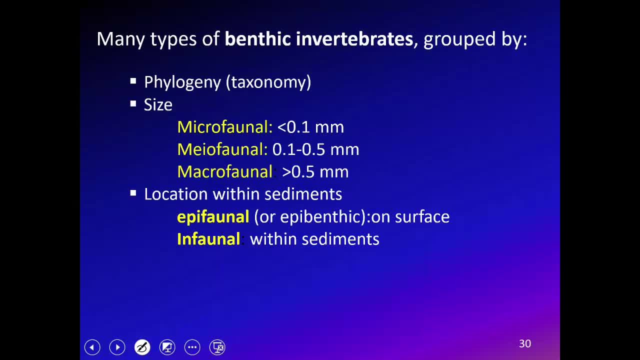 okay, so. so that's how, another way we can group these organisms by where they live: epi funnel on top of the sediment surface, in funnel within sediment surface that they they actually burl into the sediment. and then another way we can divide up these organisms is by how they get. 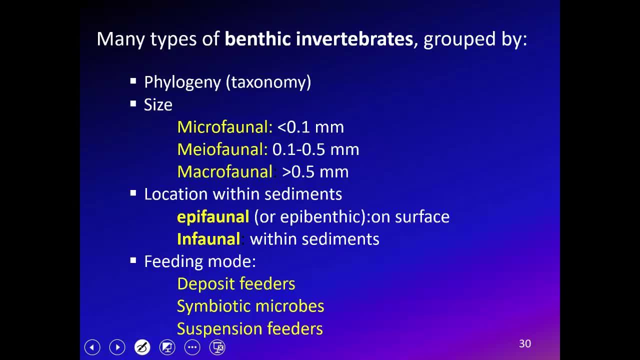 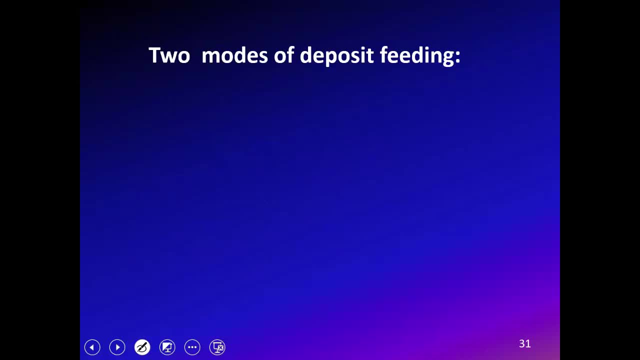 their feed, how they get their food, and we'll go about through these three types of feeding mechanisms. first, deposit feeding. well, you know what's. what's that word? deposit here just refers to the fact that they're, these organisms, are on the bottom in the benthic zone, in the benthos, and they're feeding on what's. 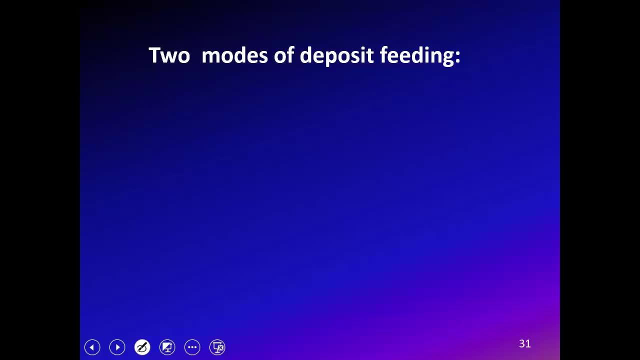 ever been deposited on them from the surface. again, remember, uh, that for the most part, the food that they get is from prime production that's occurring in the surface waters. now there are some shallow waters that are shallow enough to get enough light to support, um, in situ prime production, that is, prime production by benthic algae that are on the 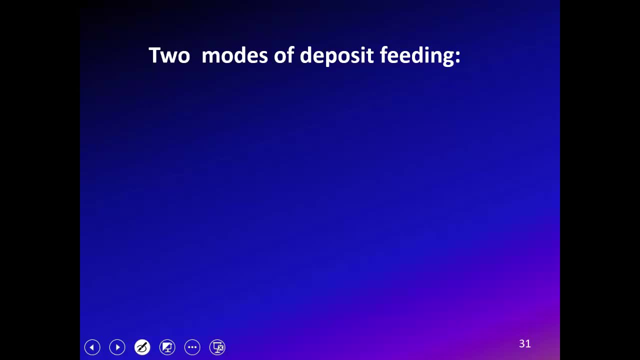 sediments themselves, but for the most part they're. these invertebrates are depending on things that are being deposited, the detritus that's being deposited on them. so that's that's the word deposit. feeding is what's used to describe these organisms. so there's two types, basically one. 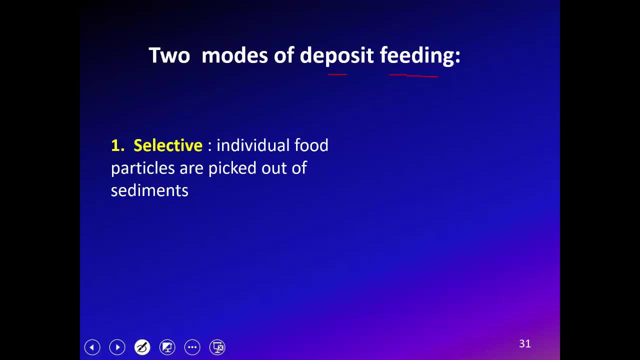 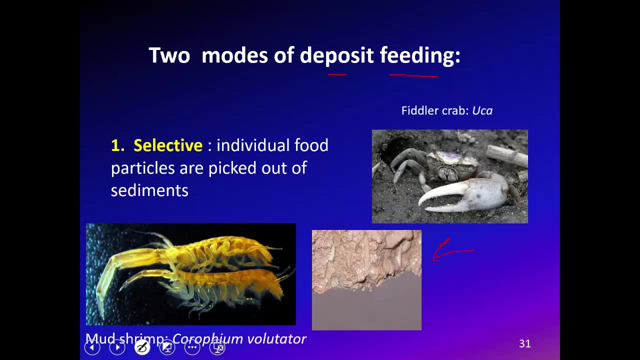 those that are picky and basically pick out individual food particles. um, here's some examples of mud shrimp, kind of an ugly looking orgasm, uh, probably not eaten very much, um, and then, uh, the one that you may have seen around on the shore is the pillow crab, and you can just kind of picture. 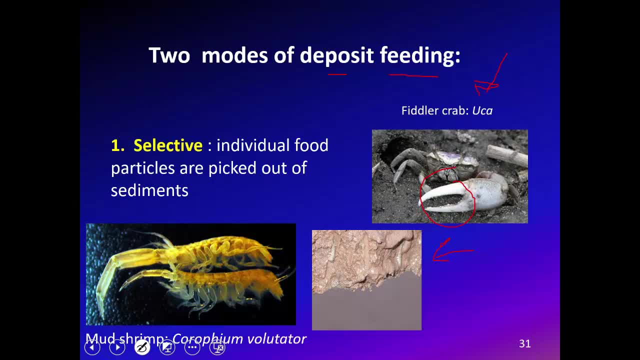 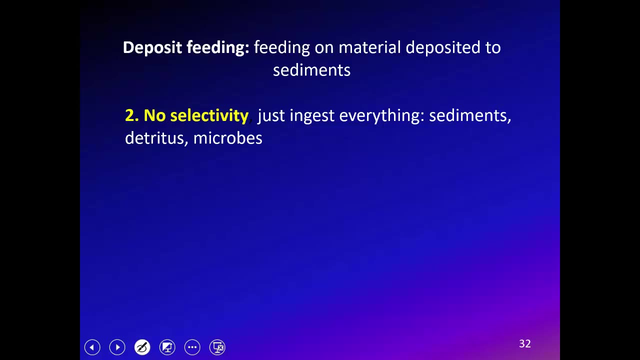 this, you know this orange and feeding with that, uh, those pincers- although i suspect that's more in defense mechanisms of that- rather than getting food. so, anyway, they're just picking things out of the sediments. um, so another uh, another, uh, a mode of deposit feeding. feeding, um, are those that do not have any selectivity, they're just. 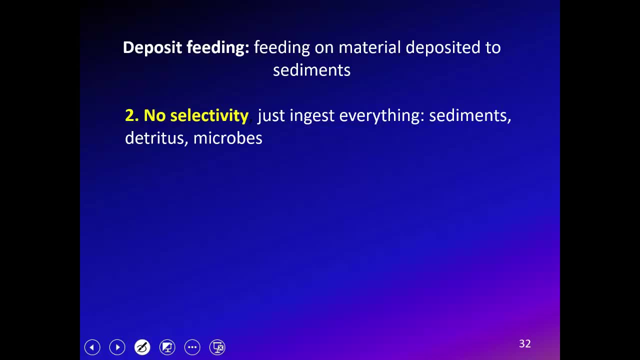 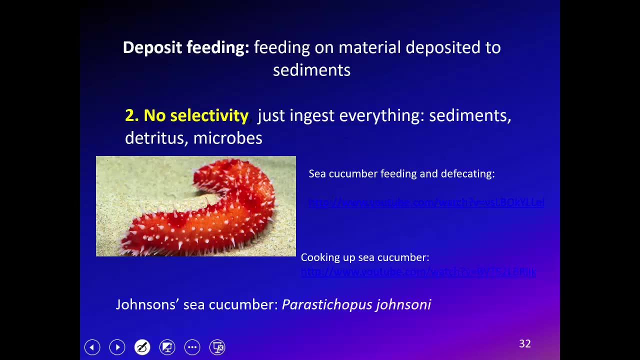 you know, shoving things in their mouth and eating everything that they can and ingesting only what they of course are are able to. to let me take that back. they're ingesting everything they can, but then they digest only that- those parts of the things that they're ingesting that are they can degrade and break down and use. 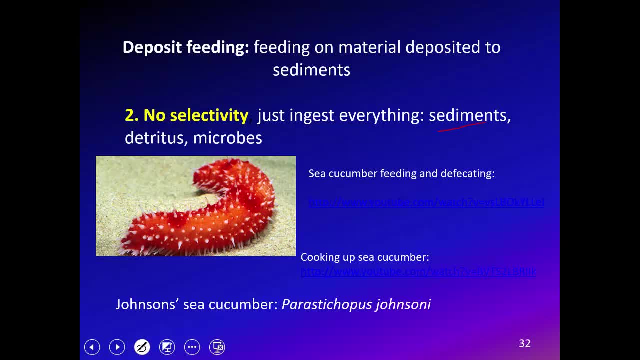 so they're getting everything sediments, detritus. so it's. i'm using the word sediments now here to to talk about the inorganic constituents. um, they're taking that in, they're taking the detritus in. they're taking in microbes that may be under detritus, or microbes are just living free. 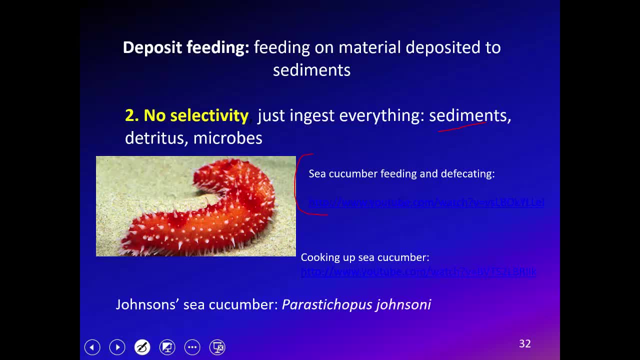 of the detritus, and so one example: that is a sea cucumber, and i'm gonna show in class this movie or you can see it yourself. it's kind of funny. i like it. um, you can see, if you want to do this at home, how you would cook up a sea cucumber. 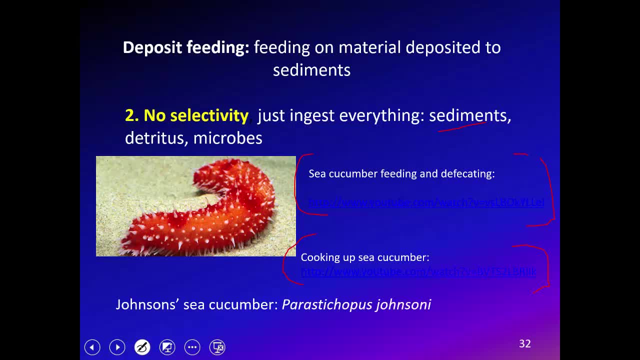 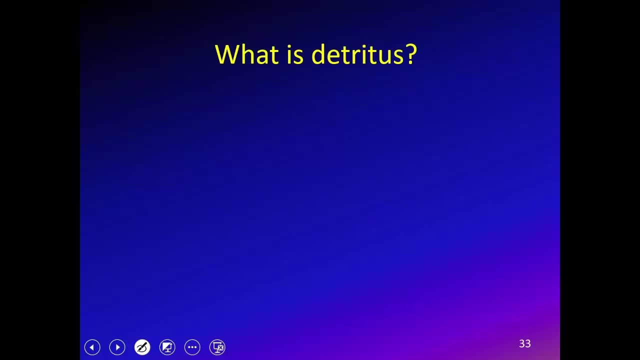 um, so, uh. so that's one example of non-selective, uh, deposit feeding. so so we've. i've been using this word detritus, and so let's spend a little bit of time making sure that you know what that word means. not a really complicated word, but it's a really 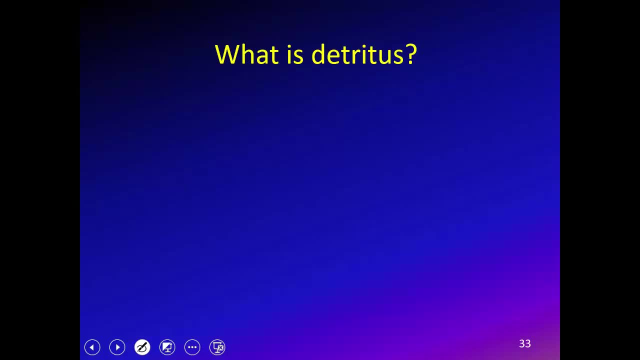 important part of what's happening down here, and i think it's one thing that's really different from, perhaps, our everyday experience of thinking about um, um organisms in terrestrial environments. these invertebrates are eating things that are not alive. That's the main, very simple definition of detritus: non-living organic material. 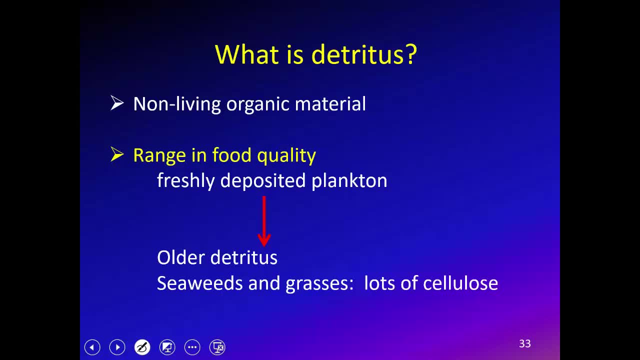 And it can range from things that are just basically not that long dead- freshly deposited plankton- to much older things that would be probably pretty hard to degrade. It has lots of cellulose, for example, and if it's near land it may even have lignin cellulose, which 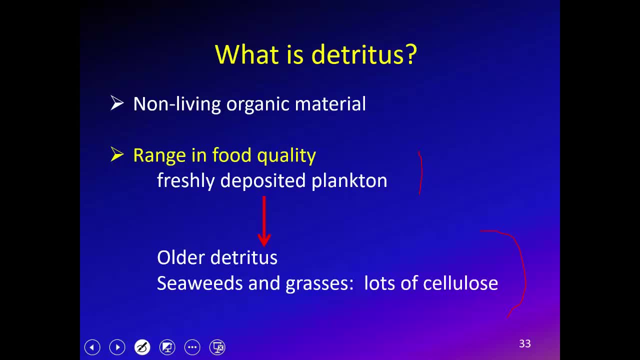 makes up wood And if you think about it, we're talking here about detritus feeders. Those are organisms that feed on detritus And if you think about it for a bit, you probably never thought of yourself as a detritus feeder. but in fact that's what you are Now. hopefully you're feeding on. 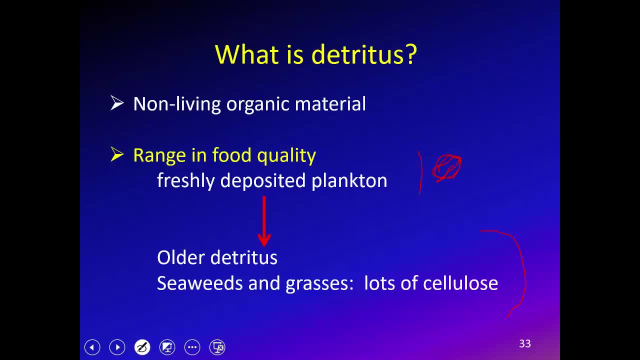 things that are fairly freshly deposited on your dinner table, That have high food quality, but with few exceptions, you're living and eating non-living organic material. right, You cooked it. Or even a salad is pretty dead. Now, if you talk about 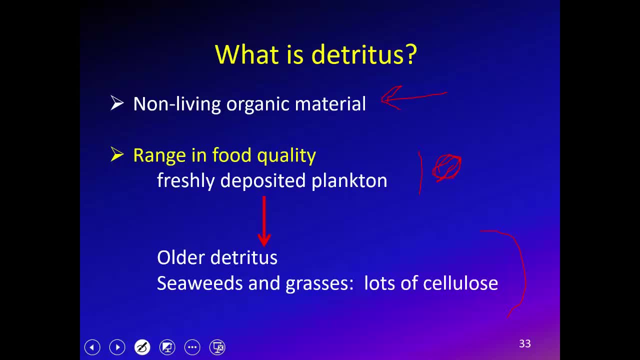 things like yogurt. you know, yogurt actually is quite, quite alive with microbes A little bit. you know, I don't want to think about that too much actually, But that's probably the only exception. Otherwise, you're living on detritus things. that's not living, And that's the case. 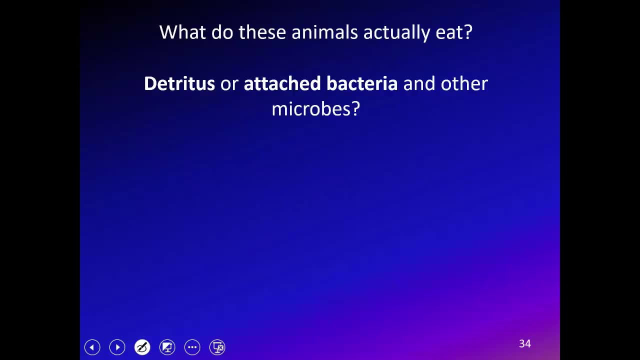 with these organisms. So, but the thing is, with these organisms, you remember, especially the ones that are just kind of eating everything that they encounter, what are they really eating? And the question really is: what are they eating? The detritus itself, the dead plant material, or is it the stuff growing? 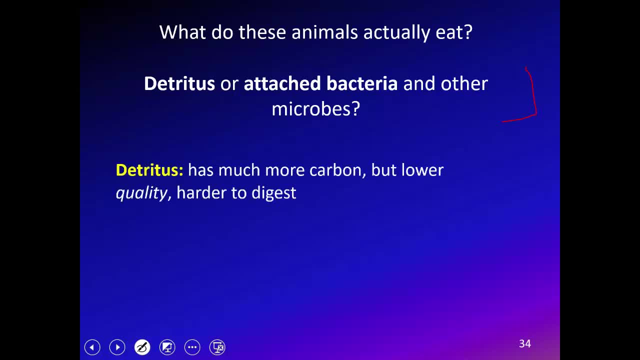 on it, The bacteria and other things that are growing on it. And the dilemma that faces these organisms is that the detritus is. there's usually a lot more of it, but it's not really good. But often it's, it's not as good stuff. Remember these micro bacteria and other small 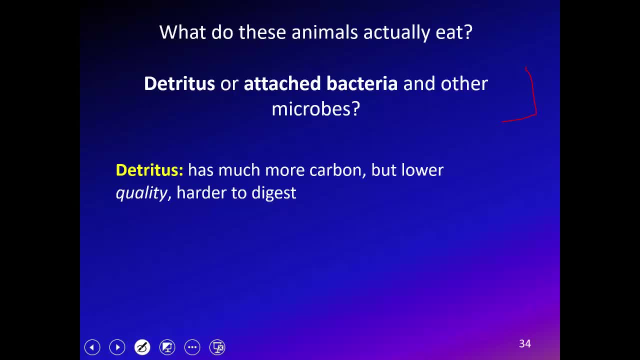 organisms are really kind of protein rich. They don't have any structural material, They don't have cellulose, They don't have lignin cellulose, And so they're really packets of protein, Whereas detritus is not that Often detritus- the reason why it's around at all. it has a bit more. 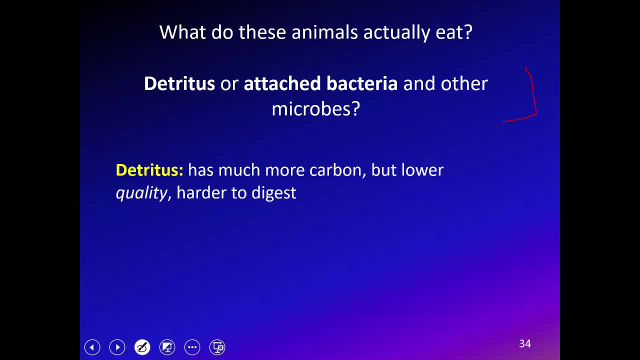 structural material, cellulose, And again, if it's near land, it has lignin cellulose, the wood. So it's not as high quality, not as high amounts of protein, But there's a lot more of it, a lot. 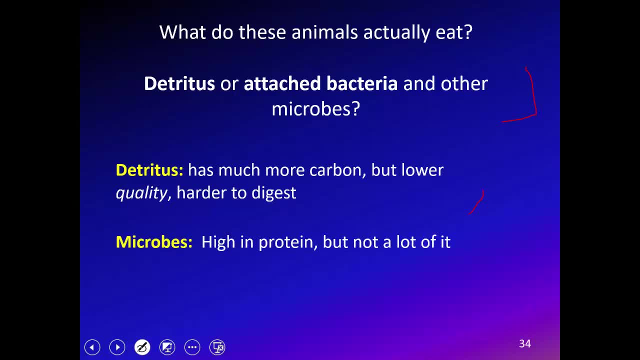 more of it. And then, as I mentioned, microbes- bacteria and other microbes are little protein nuggets but there's not a lot of it. So what do you want to go for? quality or quantity? And it's sometimes called the crackers or peanut butter analogy, And if you think about it, I don't. 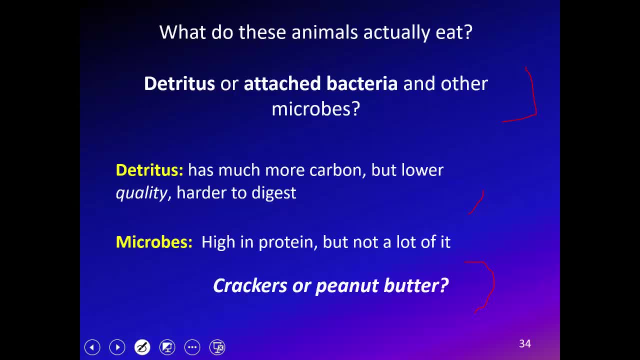 mean crackers, But one way to eat them is basically you're just kind of using the crackers to carry the peanut butter. Actually, I'm not sure why you know these deposit feeding biologists settled on this analogy. Maybe a better analogy would be cheese and crackers. I mean, crackers are just 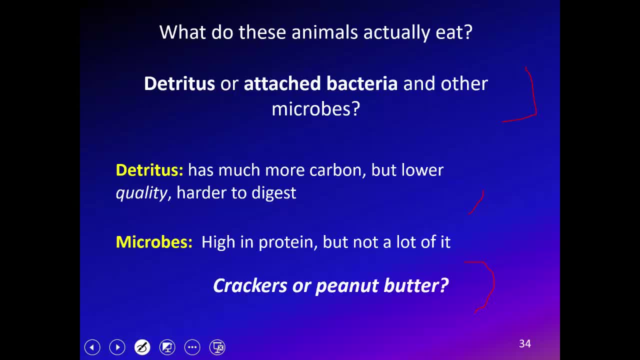 serving, at least in my case, as a vehicle to carry the cheese to my mouth. I don't really care that much about the crackers, I'm more interested in the cheese And so anyway. so in this case it's been called the crackers or peanut butter problem. 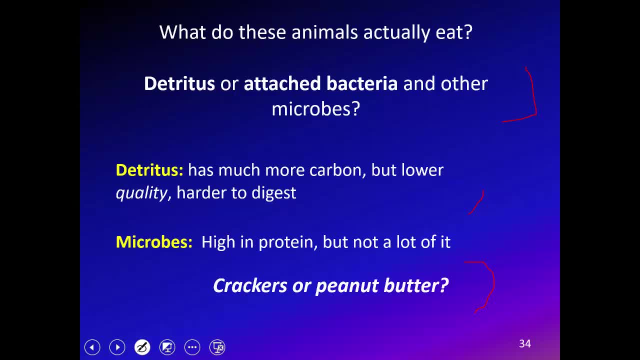 You know, are you going after your crackers, which basically is there's no protein at all in crackers. It's just a dry, boring thing to carry the peanut butter, which has the protein and a bit of fat too also. So how do you answer that? 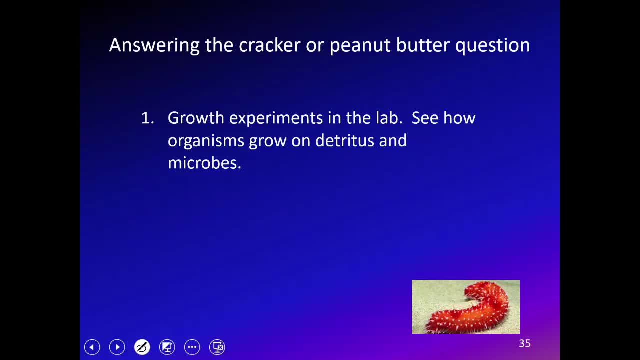 Well, one thing you do is you can grow these organisms in the lab. some of you can grow in the lab, or at least keep in the lab long enough to see what they they, they eat, and see which one to grow, And then you can see whether it grows better on, whether it grows better on detritus or microbes. 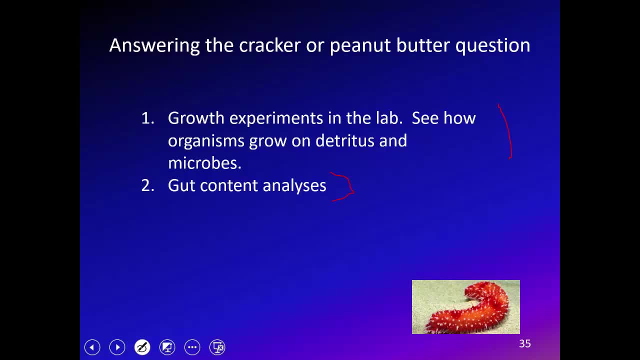 Another way to answer this question is: you look at their guts. So anyway, to back up, the problem with the growth experiments is sometimes it's hard to get them to live in the lab to do that experiment. hard to you know, get the right detritus and to do an experiment that really mimics what happens in nature. 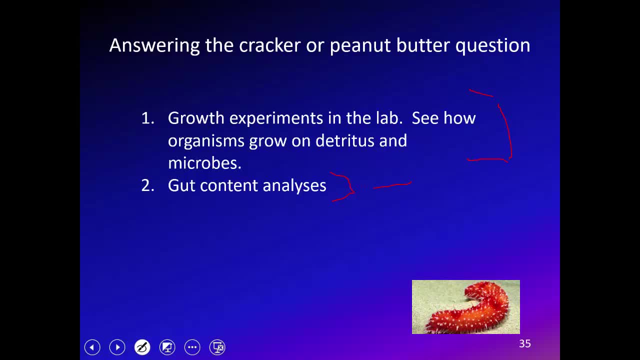 So that's not a perfect way. Another way is you look at what's in their guts. This is a very common approach to looking at what animals feed on. is you just basically open them up or somehow get their guts and look at that? Now, immediately you probably recognize. or, if you thought about it long enough, you realize that by the time it reaches an animal's gut, it may have lost any shape at all of what's actually. you know what was the original food. 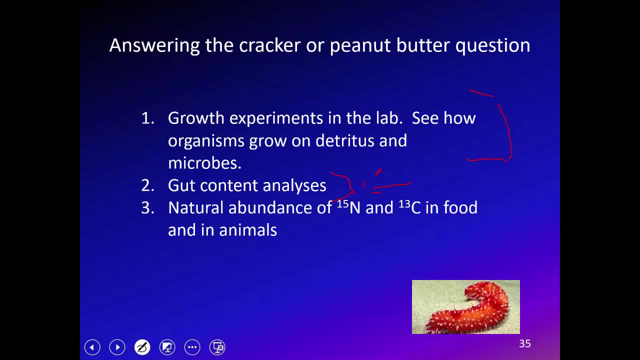 So that's not a great Great way of doing it. And then some other ways are a bit more sophisticated and we'll spend a bit more time on that. One is to use a natural abundance of M15 and C13. These are just naturally occurring isotopes that we see in the possible food for these organisms. 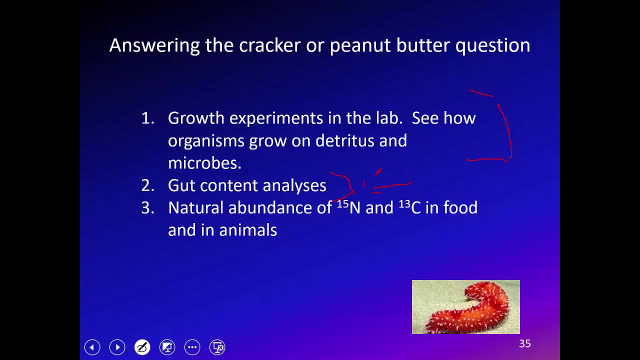 And there's ways in which you can deduce what they're eating from the natural abundance of these two isotopes. I can't say anything more about that. I want to say a bit more about experiments. Now, this is, this is where what you want. 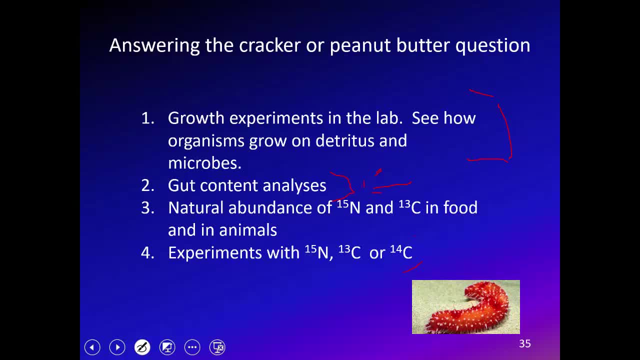 What you're doing is you're labeling up food with these isotopes. These are two stable isotopes are not radioactive- C14 is a radioactive isotope of carbon. So basically, what you do is you feed. I'll just stick to the stable isotopes. 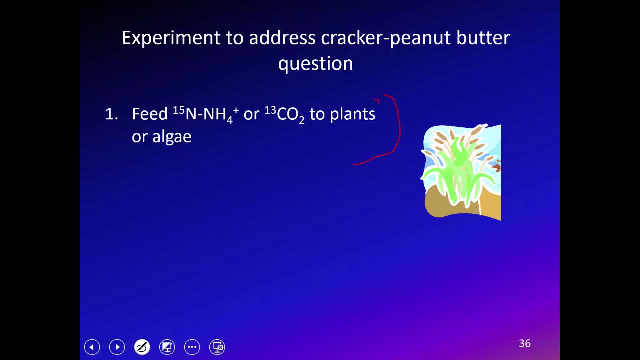 You feed to plants or algae in order to make the detritus either M15, ammonium, or C13, carbon dioxide, And so then you're making that detritus from plants Or for algae. that's now labeled with those stable isotopes. 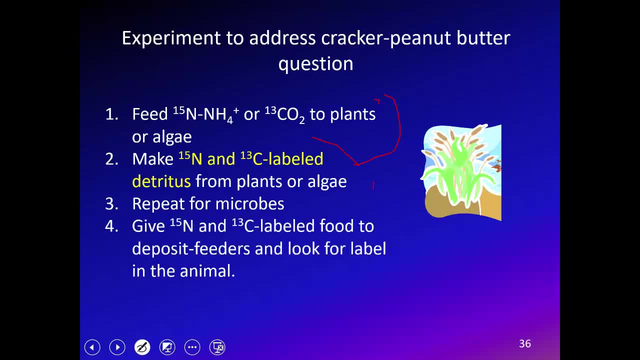 And then you do that also for the microbes, And then you feed that now labeled food back to the deposit feeders and look for the label in the animal. So the advantage of this: you can do this in a relatively short term experiment. You can do it in conditions that perhaps mimic more closely to the natural environment of that animal as opposed to the lab. 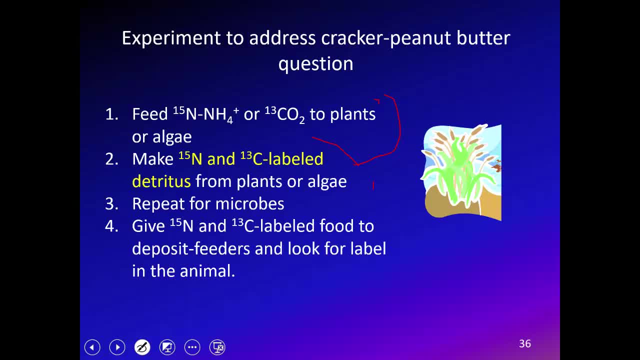 It has its drawbacks, but is a very powerful approach for looking at this question. And the answer is: well, as you may guess, it depends. It depends on the deposit feeder and depends on the detritus, And I have to say, for the most part, they're getting most of their carbon from the detritus. 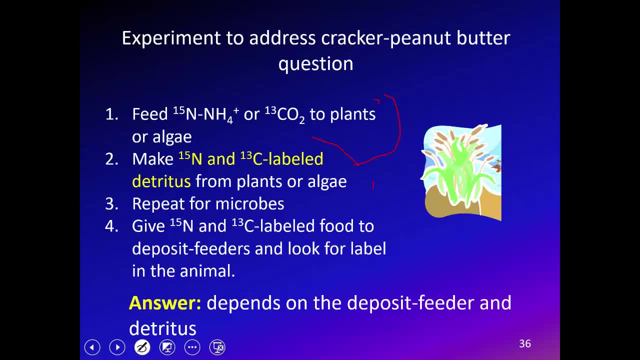 And they may be getting some of their nitrogen from the bacteria, But overall it depends. You know why am I showing you this? The point here is to show you experimental technique For getting an important question about the metabolism and feeding strategy of these organisms. 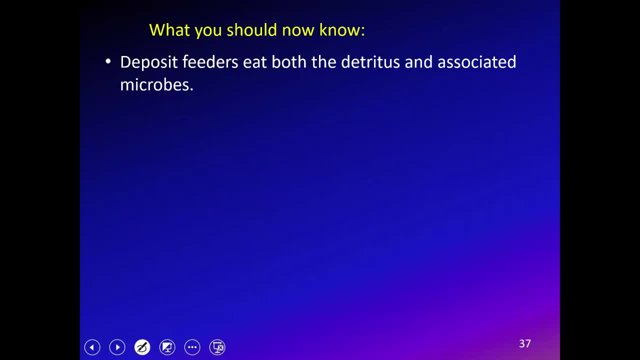 Okay, So you should know now what deposit feeders are and the fact that they eat detritus and associated microbes. You should know that these invertebrates- as we've seen for all the invertebrates encountered so far, can be grouped and classified not only by taxonomy. 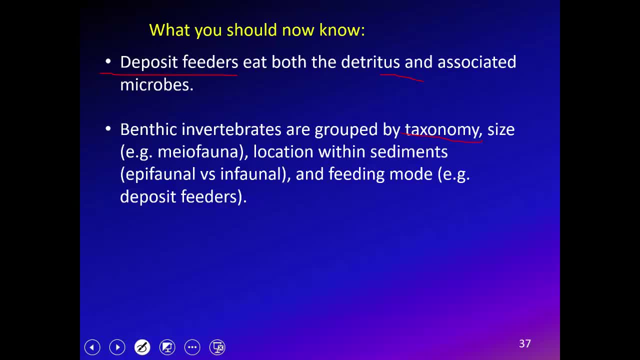 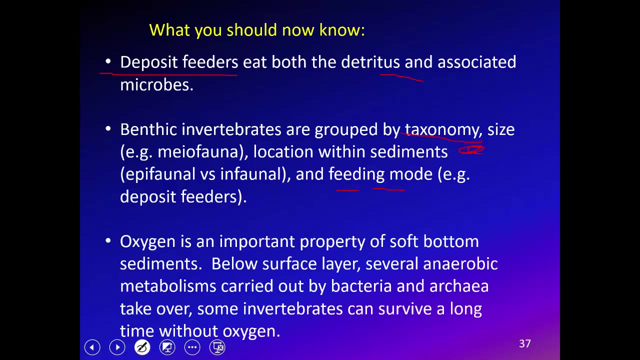 Okay, But by size. And in the case of these imbentic invertebrates, you can talk about them, about where they live, epiphaunal versus infaunal- And finally their feeding mode, one being deposit feeding. And the other point that you should know now about these soft bottom sediments. this is not really an issue with hard bottom sediments. 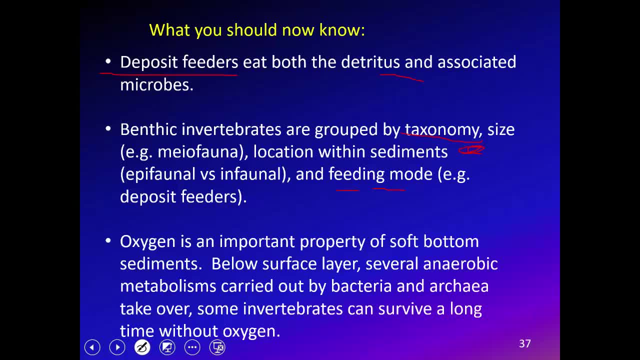 First of all they're hard. There's no nothing to get into into a rock. Okay. But also with these with harder sediments, with, say, gravel, there's just not enough organic material to use up all the oxygen. And in soft bottom sediments oxygen disappears within a few millimeters and anaerobic metabolism take over. 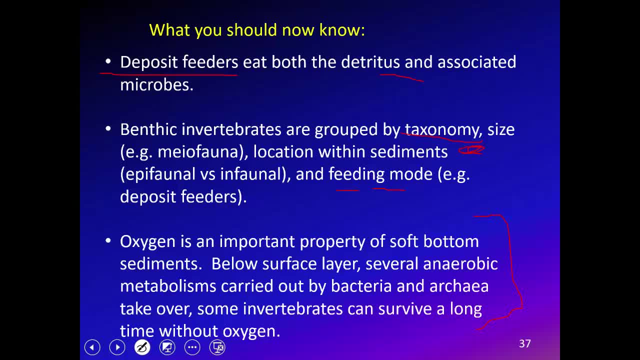 For the most part dominated by these microbes, bacteria and archaea, Although there are some invertebrates that can survive Long times without a long time without oxygen, And that's a topic we'll get into when we talk about the dead zone problem that we see in coastal waters around this country and also elsewhere. 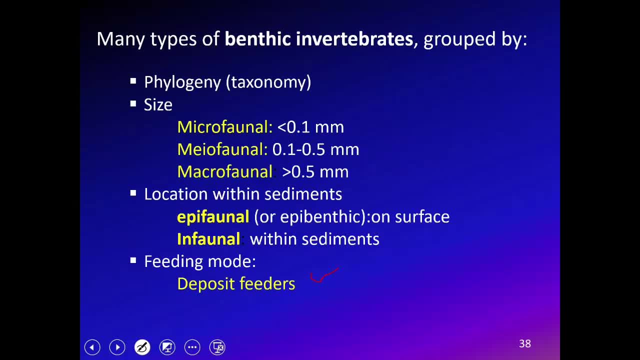 Okay, So we've talked about deposit feeders and let's continue on our our our survey of other types of marine benthic invertebrates that feed by other mechanisms, And the other mechanism is is to rely on the microbes. 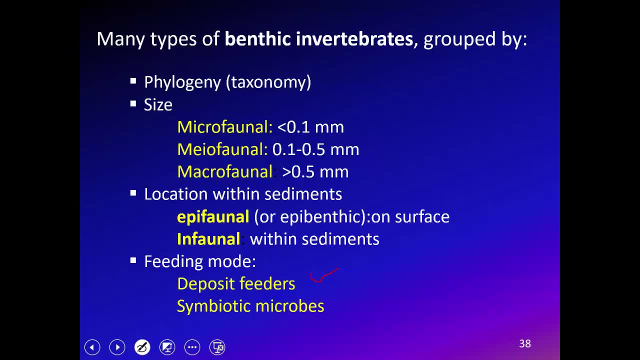 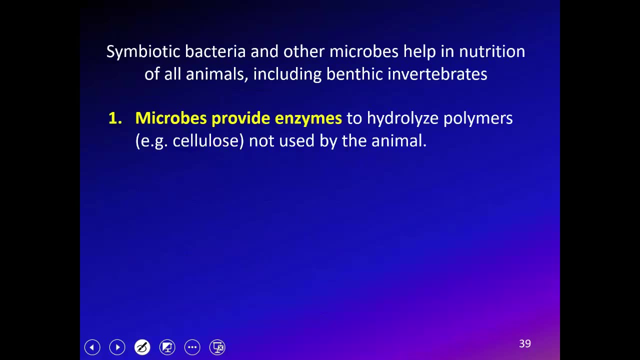 And these are symbiotic microbes, microbes that are occurring with, living with these invertebrates and helping them survive by using compounds that the invertebrate cannot otherwise use, And so the types of symbiosis vary quite a bit. It can include microbes that provide enzymes to degrade and hydrolyze polymers that are not used by the animal. 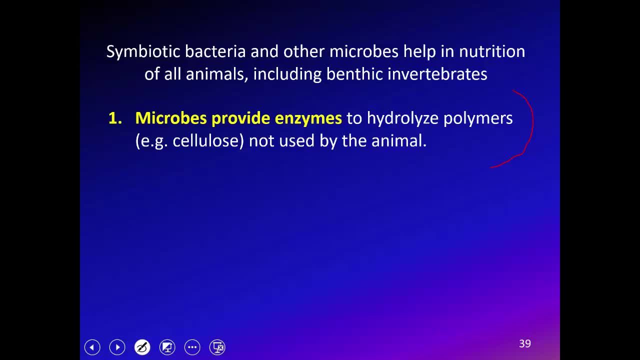 This invertebrate. This, in fact, happens with us as well. We have symbiotic microbes within our digestive tract that help us digest our food, And that's certainly the case with several animals and invertebrates where they cannot degrade, for example, cellulose. 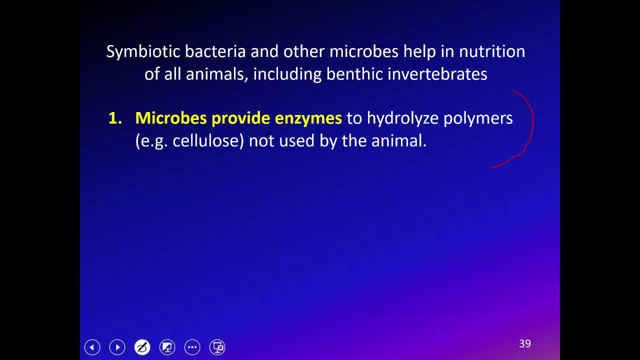 And it's the microbes that are doing that hydrolysis, that breaking up of that polymer into byproducts that can be used by the animal. But the example that's seen where, The example that's seen with these benthic invertebrates- which is really spectacular, I think, and really unique- and we don't see that with us for sure- is, is these chemolithoautotrophic bacteria that are using compounds that otherwise the animal cannot use. 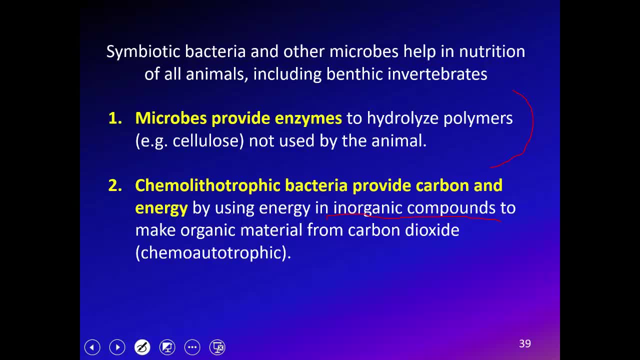 And they're getting energy from these inorganic compounds and making organic material, like the phytoplankton analogy that we've seen already- And and that Organic material is, in turn, used to feed the animal. So we'll say a few more words about that. So the full name is- and I've used it already- is chemolithoautotrophic bacteria. We're going to see this again when we talk about hydrothermal vents, But I want to mention now, in this case, in this, in this lecture, because it is an important example of of how these invertebrates make a living. 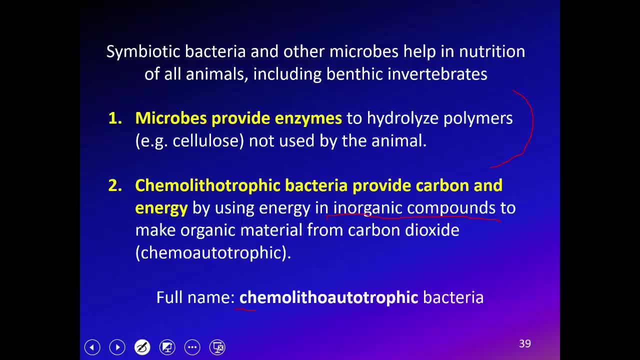 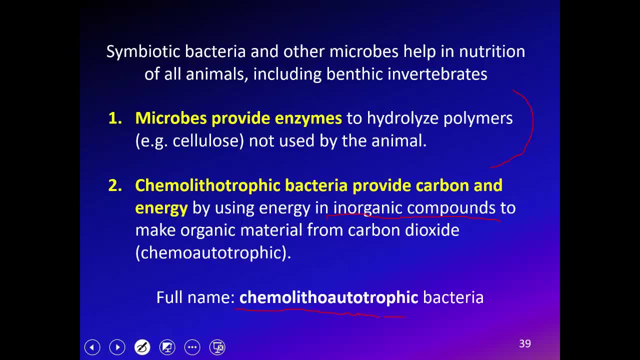 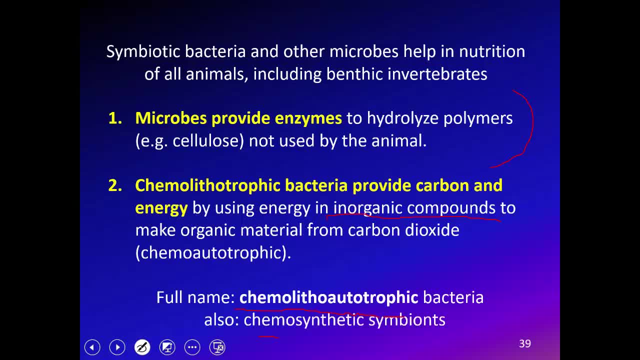 Chemosynthetic, Chemosynthetic, So so another word that's used for this is chemosynthetic. I think it's not as useful, Because on the their the word that's used in this case for these chemolithoautropic bacteria. 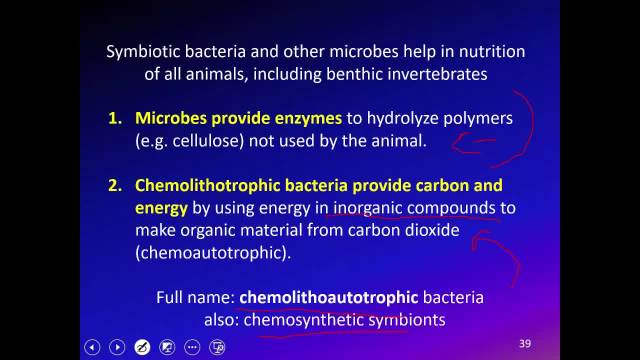 But not in this case, where the microbe is just is is helping as much. It's also chemosynthetic, But it's just not doing what these organisms are doing, So I'd like to stop. The word chemosynthetic is only used to describe these chemolithotropic bacteria. 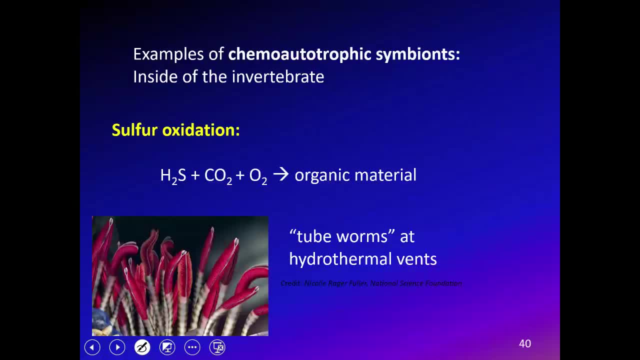 Okay. so what's happening here is that is a use of this otherwise very toxic compound. hydrogen sulfide is used as an energy source by these chemolithotropic symbionts, And they're using CO2 as their carbon source and they're making organic material. 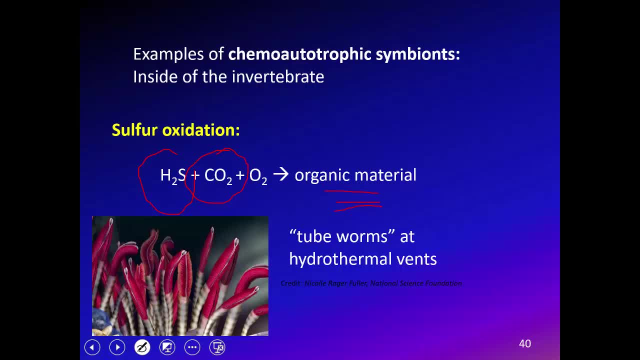 They're making organic material for itself, They're making more cellular material and that cellular biomass of the bacterium then goes on to feed the invertebrate And a spectacular example of that is tube worms that we see at hydrothermal vents. So in the third course, third, I think I don't think we're, I can't remember now if we talk about hydrothermal vents. 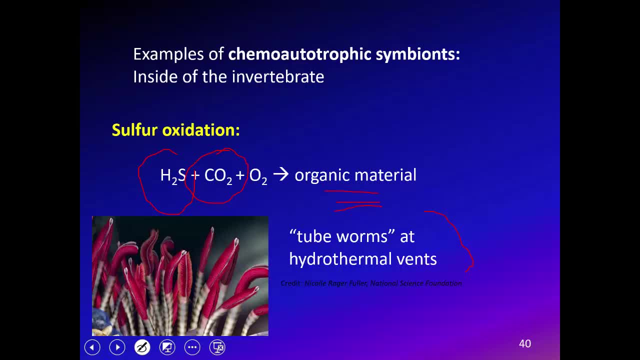 this third of the course, or the final third, But anyway, we will be talking about hydrothermal vents Soon and we'll see more about these chemosynthetic symbionts that occur within the tube worms, that hydrothermal vents, And we'll talk a lot more about vents as an ecosystem. 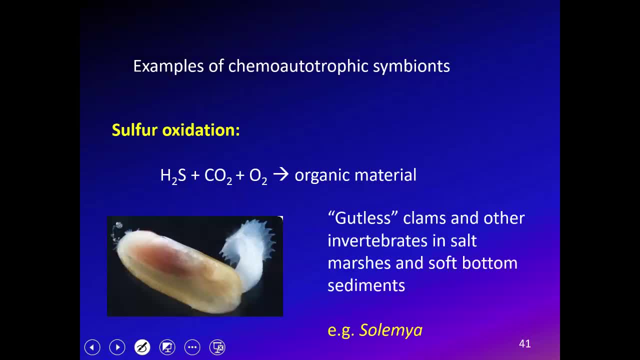 But? but these also occur much closer to home, in salt marshes that are just in our backyard. here, at least down here in Lewis, There are some types of clams that don't have a gut, they don't have any digestive tract And they are relying on these chemo autotrophic symbionts to again carry out this reaction of using the hydrogen sulfide that's produced by that sulfate reducers that are, these hydrogen sulfide oxidizing organisms, are fixing CO2, making again organic material, more biomass for itself. 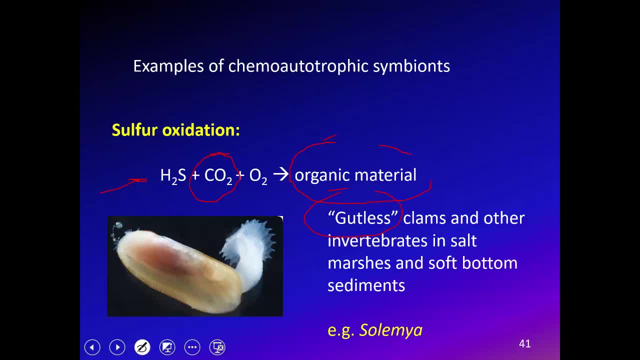 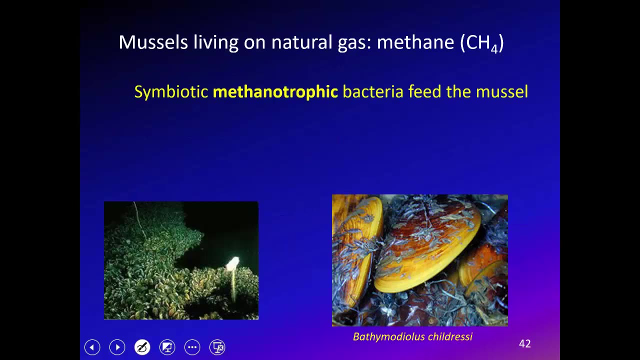 And that organic material then goes on to feed these clams and other vertebrates that have these chemo autotrophic symbionts In this. So that's a great example of how symbiosis is helping these organisms. And the final example is: is perhaps I don't know what's more bizarre using hydrogen sulfide, a toxic gas, or methane? 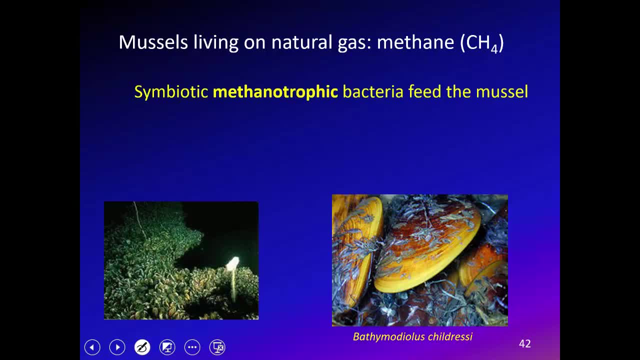 There's muscles that live on natural gas, and they live on natural gas thanks to the work that's been done by these methotrophic bacteria, and methotrophic bacteria using the methane That's Coming out of what are called cold seeps in the Gulf of Mexico. 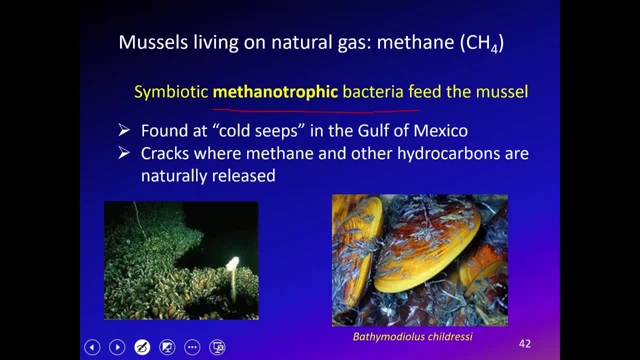 And elsewhere a couple of places elsewhere in the world. So cold seeps are basically places, cracks in the Earth's crust where methane is is getting out and other hydrocarbons. So you probably know that there's lots of oil deposits in the Gulf of Mexico. 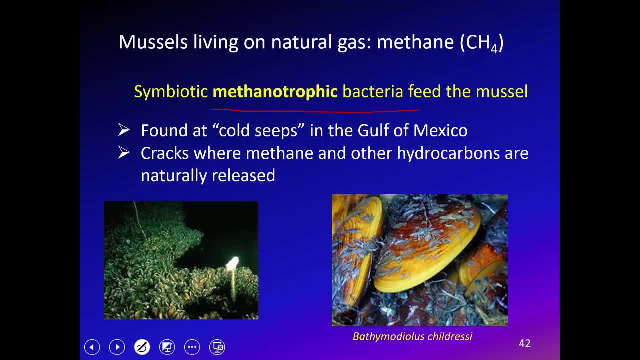 That's why we have oil derricks out there to drill for oil. What may not be quite as obvious is that Even without those oil derricks out there and in in drilling, there would be methane oil leaking out of the the bottom of the Gulf of Mexico. 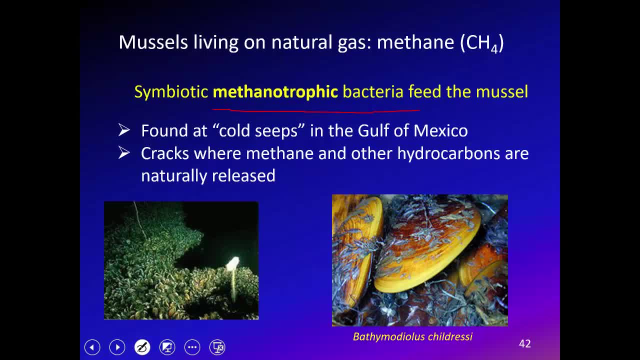 And there's organisms that take advantage of this energy. rich suite of compounds are coming out. It's only bacteria that can do that, And and muscles have figured out how to some muscles have been able to figure out how to make use of these bacteria and 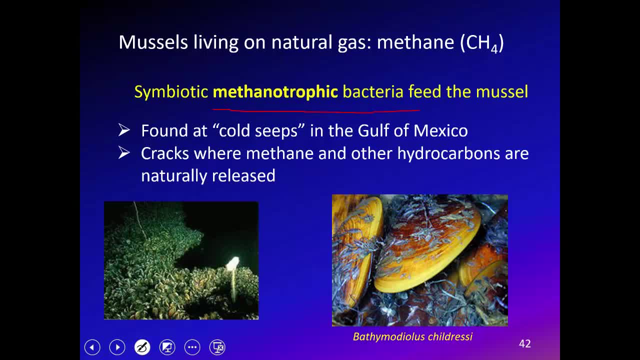 And the symbiotic relationships. So the so it's: the bacteria again- are using the methane as a carbon source and as an energy source, And the bacteria are making organic material for its own bodies, And then that organic material then goes out to feed the muscles. 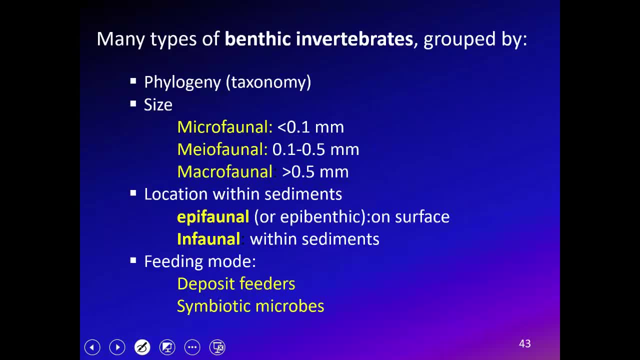 There's an example of that here. OK, so that's that. there's a. we're going to say a bit more about the hydrophilic event animals, but that's all the time we have for symbiotic microbes. And now we're going to go to our last form of of feeding, and that's called suspension feeding. 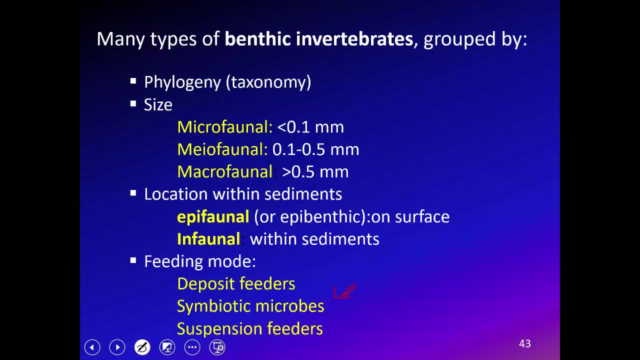 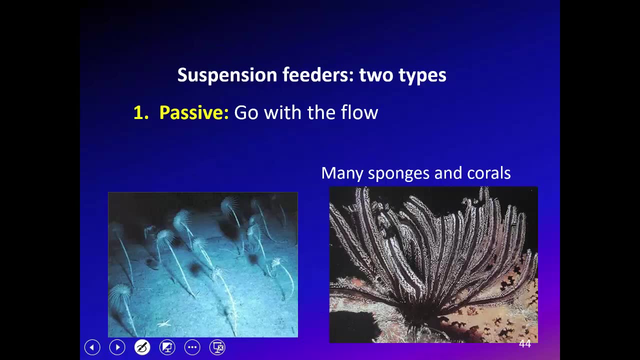 So suspension feeding is somewhat like filter feeding, is very much like filter feeding, But the word suspension feed- feed feeders are- is used to describe those benthic horses, as opposed to this old plank that we talked about earlier for filter feeding. So the suspension feeders can be divided into two types: one that basically are are just kind of sticking their little arms out, or 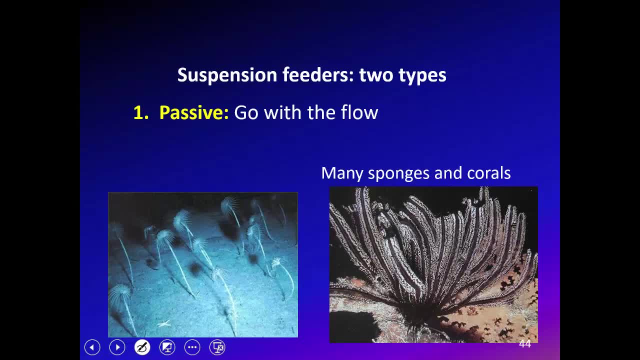 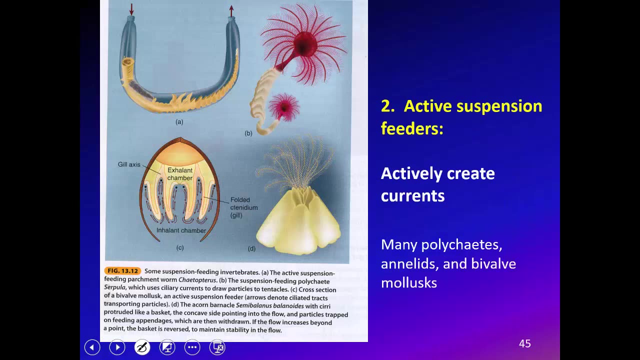 Are feeding apparatus out into the currents and just relying on the currents and water movement to bring food to them. So that includes sponges and corals as our, our animals that are used suspension feeders. Active suspension feeders, on the other hand, create their own currents. 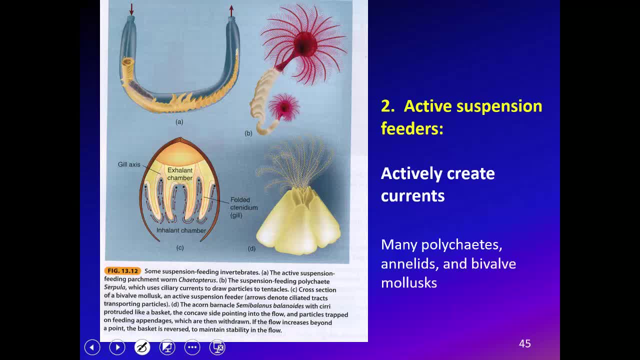 So they're pulling in water or not, or somehow creating currents past or feeding apparatus To to harvest food, and that includes, you know, you can see here many polychaetes, worms and bivalves do this type of feeding. 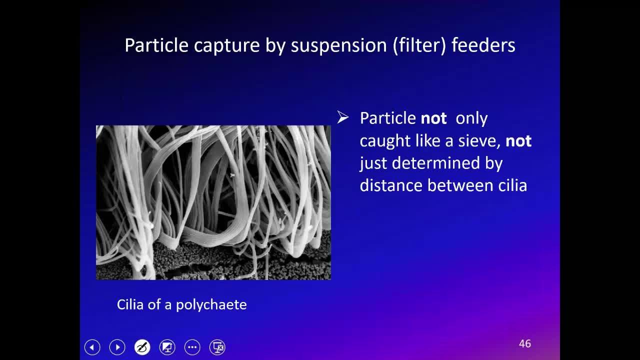 So what's happening here is is is analogous to what we saw already for the filtering feeding zooplankton, in that the particles are caught by these hair like structures, and the word that's used here is cilia and not CTA. These, these are a bit coarse. 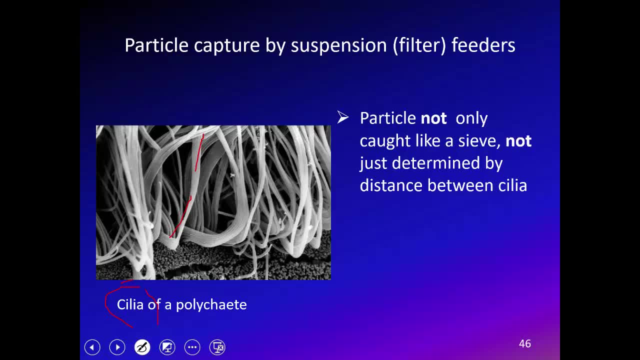 They were we saw for the zooplankton, But again the same type of physics are involved, in that the particles that are caught are are are even smaller than what you think would be caught if you'd looked at only the distance between the cilia. 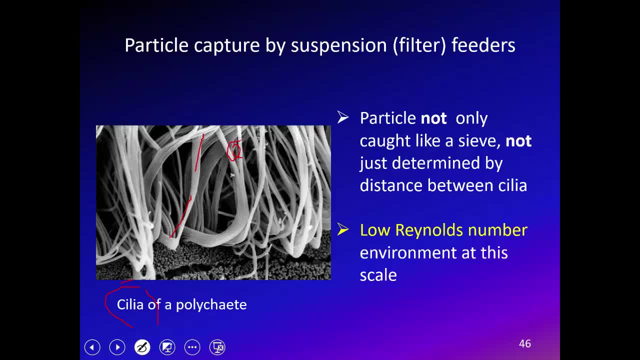 And that's again because the the environment here is a low Reynolds number- environment and the water at this small scale, which is, you know, microns and at is is that the micron scale is- is more like molasses. it's very viscous. 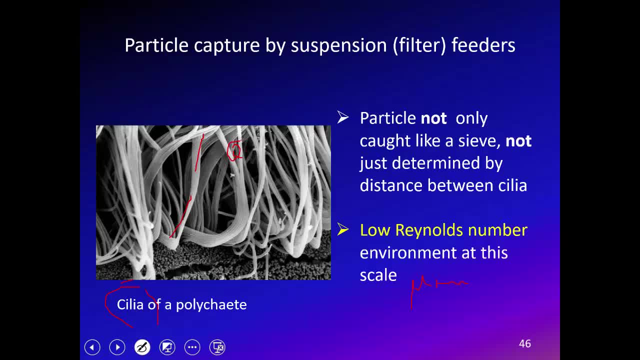 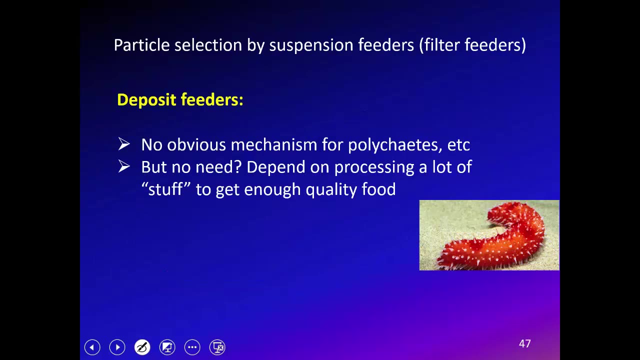 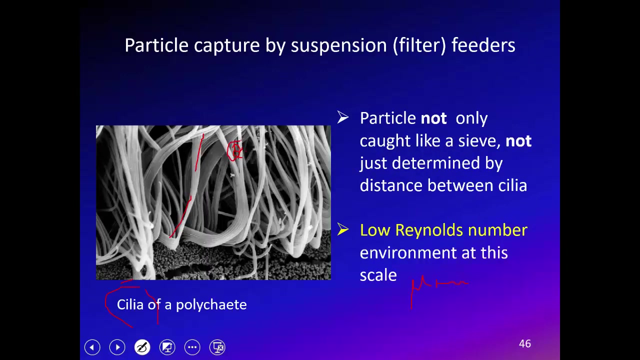 at that scale, and so these particles are trapped much more easily than one. what you expect if you just look only at the distance between these, these cilia? so that's suspension feeding. now one question that comes up is is whether there's any selection by suspension feeders. so, as we talk about for the zooplankton, you kind of know the answer already. 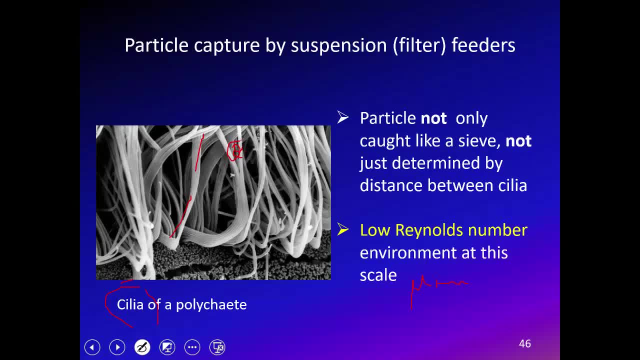 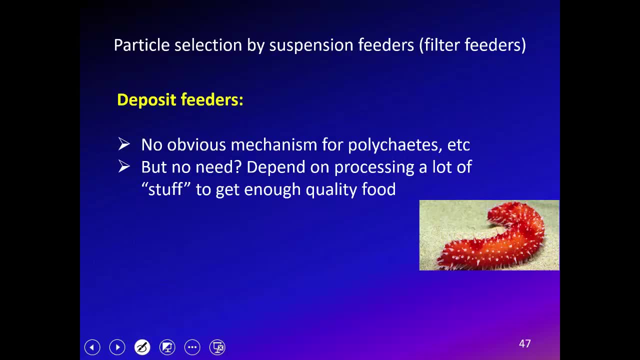 the answer basis is mainly size, that these organisms are filtering out particles of a particular size. but as we solve with the zooplankton, the question comes up is whether they can do some selection as well. that is, would there be any selection of, say, a high quality particle alga, for example, as opposed to a low quality? 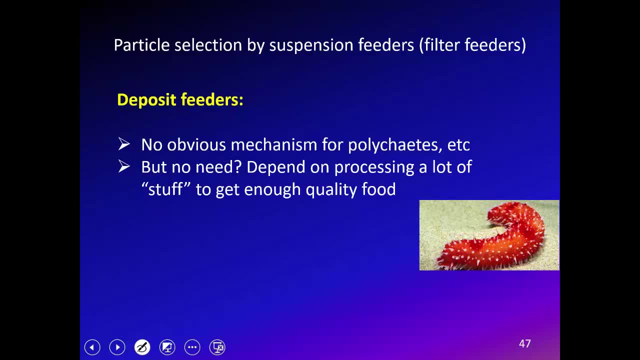 piece of detroit. this you know. they are the same size. so if we think about this, in comparison to deposit feeders, going, going back to these organisms that are feeding at the bottom, you know, through, going through the sediments, there's no mechanism, there doesn't seem to be any way and arguably they don't. 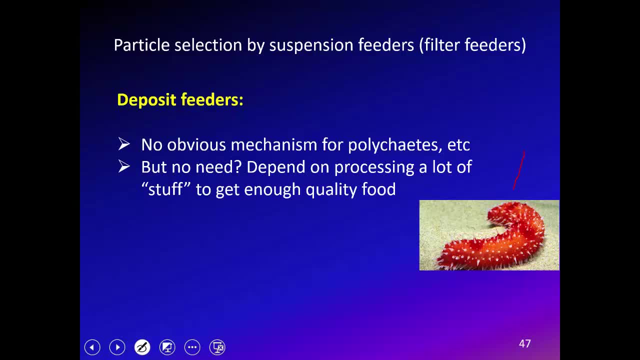 need it. so what they're doing, you know, here's the, the sea cucumber. they're basically going through the same things that they're feeding on the other side of the surface. so they're just drinking from the other side of the surface and they're really low quality and depending and they're 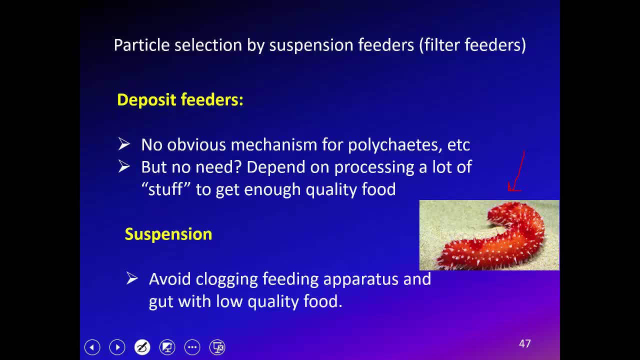 and they're kind of relying on just the quality and the quantity of things that they're processing to get enough high quality food. now, think of that. in contrast, the suspension feeder: you have these guys waving out their appendices there and they're trying to, you know, collect things in. 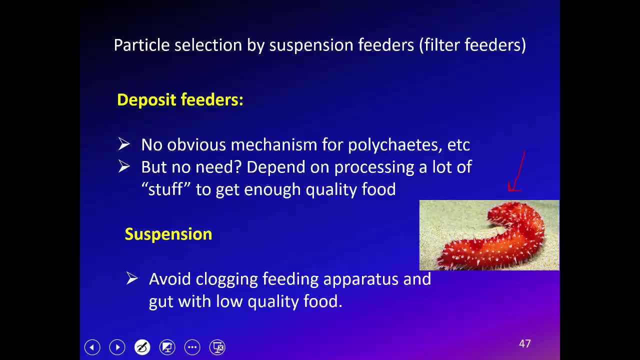 their cilia to get particles that they can feed and eat, all clogged up by things that are of small quality. So it seems like there would be more selection, for I shouldn't use selection, but more advantages to be selective in what you eat if you're a suspension feeder as opposed to a deposit. 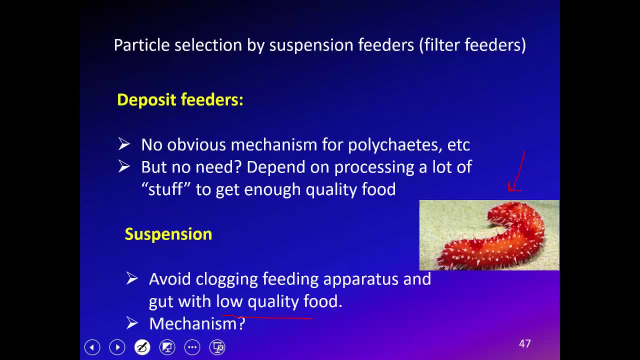 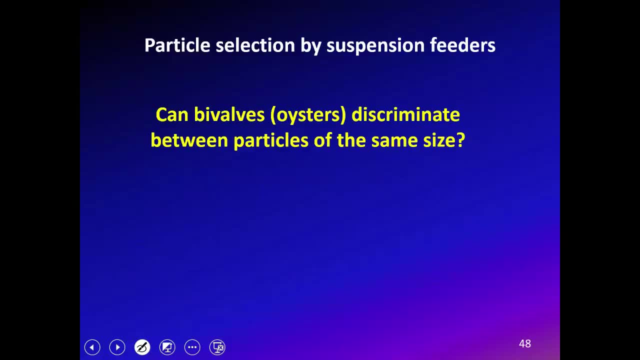 feeder, And that seems to be the case. The question then becomes the mechanism. We talked a little bit about selection by chemical cues And here by mechanism. what we're really talking about is where the selection actually occurs and what part of the animal actually does it. 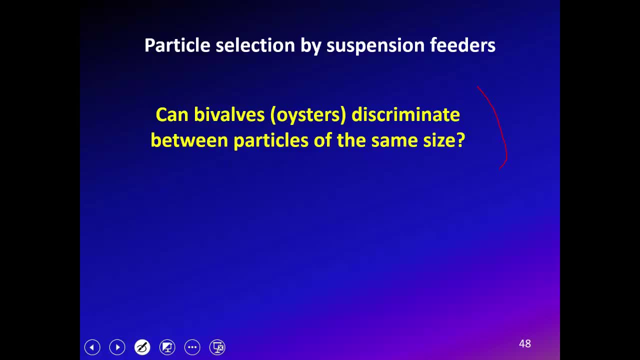 And we get, I guess, back up and say, does it happen at all? And, as you may guess, yes, the answer is yes. So the experiment was to. and here again is a case of where the actual outcome of the experiment is perhaps less important than thinking about how they did it. 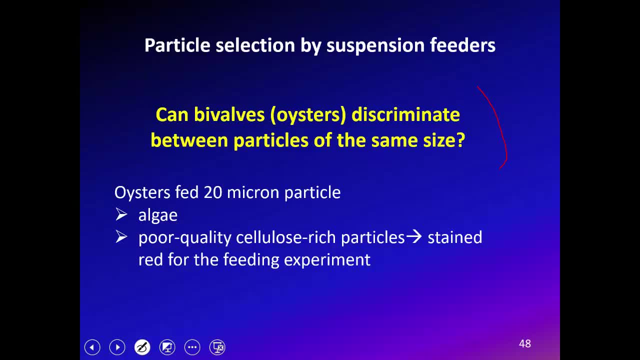 And so it'd be more. you know I hate to talk about what's going to be on the test, but a good question on a test would be thinking about an experiment to test this idea about whether they can distinguish between particles of the same size or not. 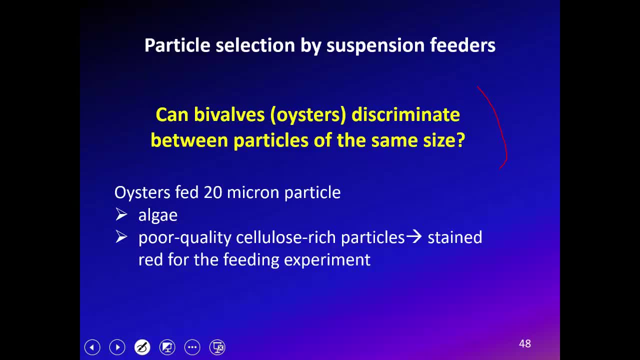 So in this case the experiment was to feed this oyster algae that are about 20 microns in size, and then also the particles that were about that same size but basically were just cellulose, You know, just little bits of grass. 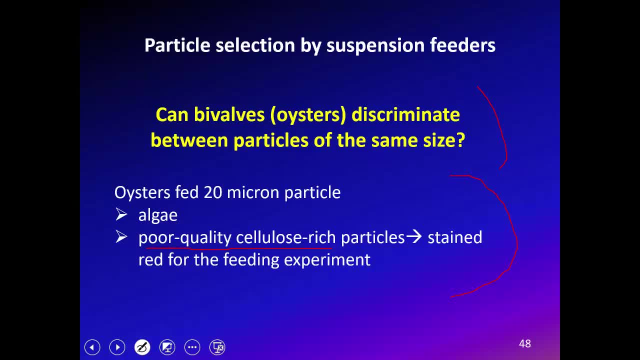 Cellulose is again the structural polysaccharide that makes up the cell walls not only of algae but higher plants as well, And algae, though, in addition to having those cell walls, would have a lot of protein and other things that make them more nutritious than just cellulose. 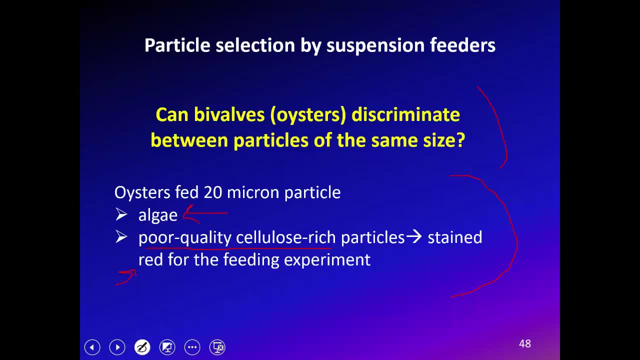 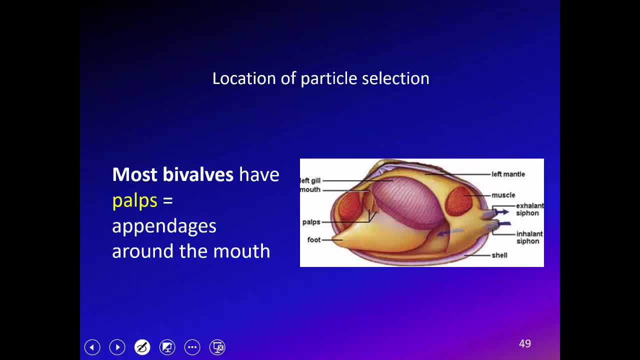 So these low quality particles were stained- with a red stain, So they could be stained, So they could be stained. with a red stain, So they could be stained, So they could be stained, So they could be stained. Now, the hypothesis was that the particle selection would occur at the palps. 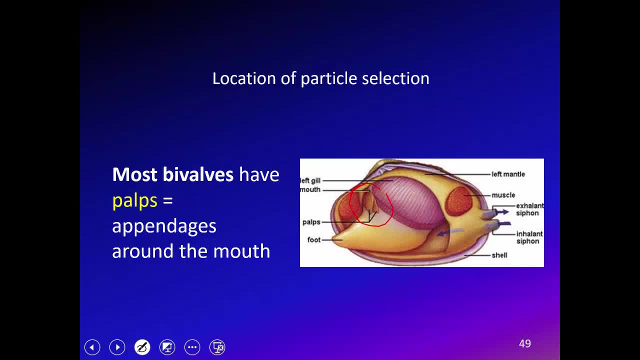 So the palps, are these like appendices, right near the mouth of the animal. So you can see, here's the mouth And so these are these lips that look like kind of appendices that are right next to the appendages- I've been saying appendices- appendages right next to the mouth of the animal. 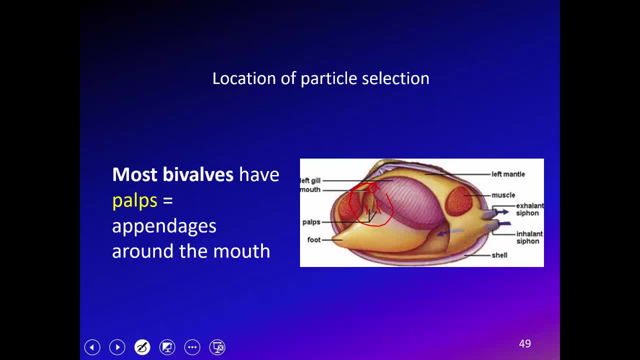 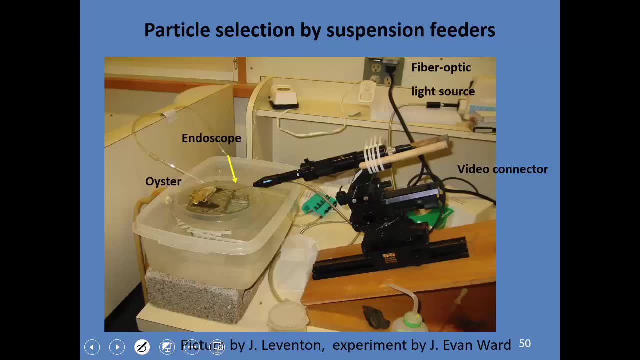 animal that were thought to be the place where food was selected, And is that the case? So that was the experiment. So the experiment consisted of looking at for the what was happening to these low quality particles that were stained red, and they were actually looked at by an endoscope connected. 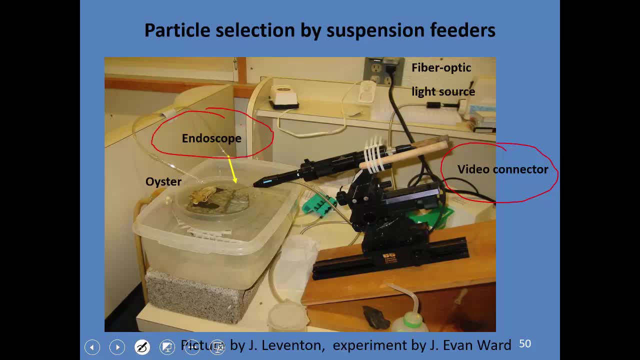 up to a recorder and an endoscope. you know is basically a small, very small camera And the experiment was done by Evan Ward. and one reason why I'm mentioning this, because Evan got his PhD here at the University of Delaware with Nancy Target. 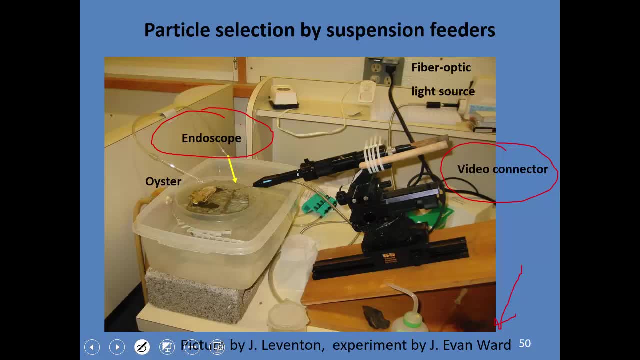 Nancy Target was the before. she was president of the University of Delaware, acting president for a year. She was a professor. She worked down here in Lewis and worked on- actually she's more of a chemical ecologist- and some of the things that Evan worked on here. 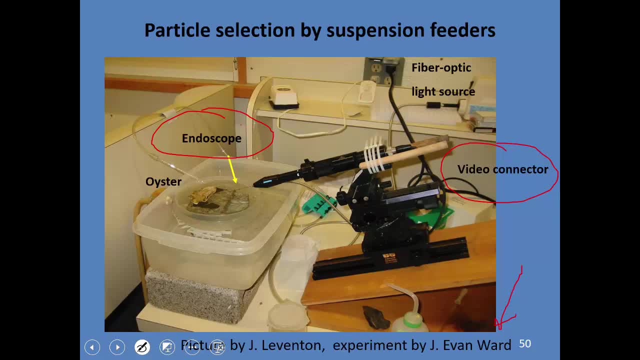 But anyway, Evan was a student of hers here and now is a professor at the University of Connecticut And I believe this work was done while Evan was at the University of Connecticut. Anyway, he used this endoscope to basically stick this camera into the poor oyster to. 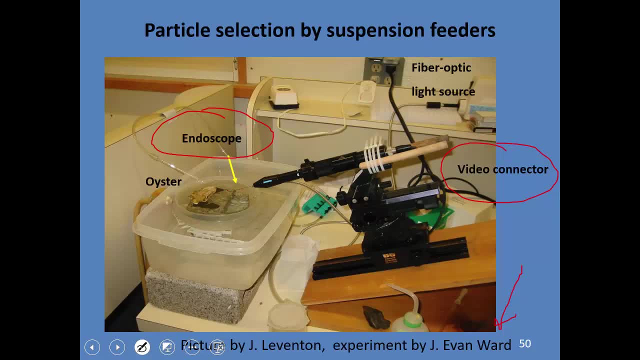 see how it was feeding- And endoscopes. Endoscopes is also used to look at our own digestive tract, and I've had the pleasure of having this stuck down at either ends of my digestive tract to see what's going on, And so, anyway, that's a common tool in biomedicine to look at what's happening within our own. 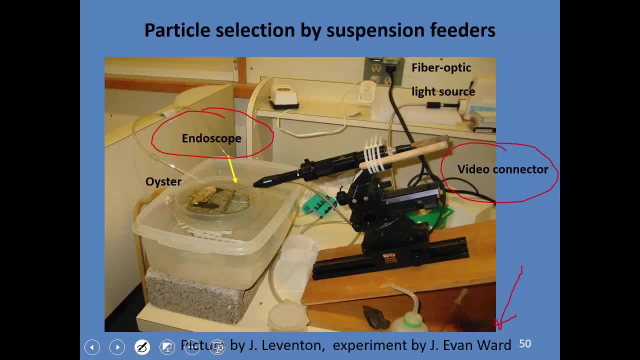 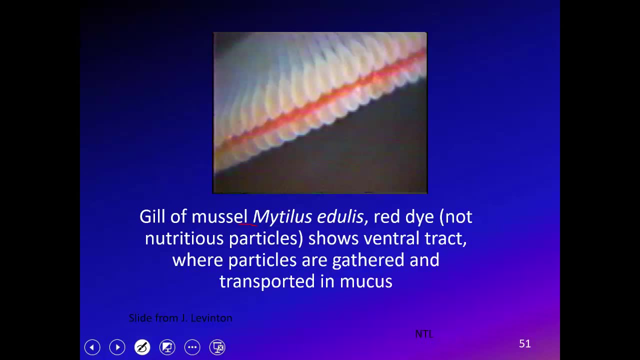 bodies And it was applied here to look at what's happened with this oyster. And here's what was done, And here's what was seen. Now, unfortunately, this was done. this picture is from a middle-ist, not oyster, but it shows. 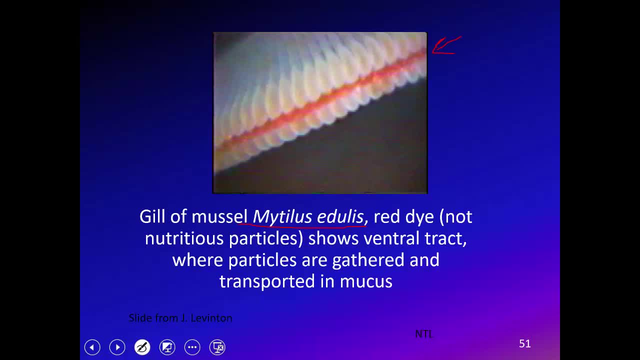 the idea And basically what's seen here is the separation of what was happening with the cellulose particles, which are not high, have high nutrition, And they are the ones that are stained red And they're shown all going down this ventral tract where they are kind of all collected. 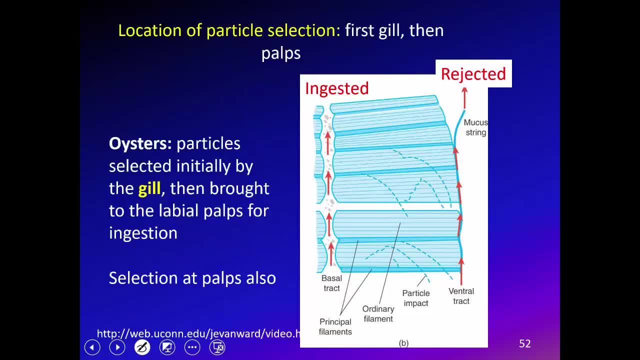 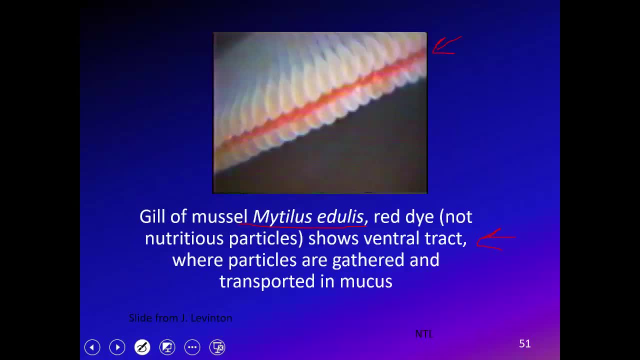 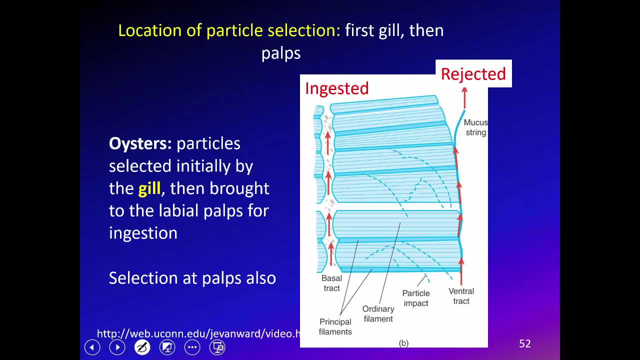 And they're excreted by the muscle, And here's the diagram just showing that. And in the experiments. so this is a gill, And so I already, before the particles were even reaching the palps, they're being selected. 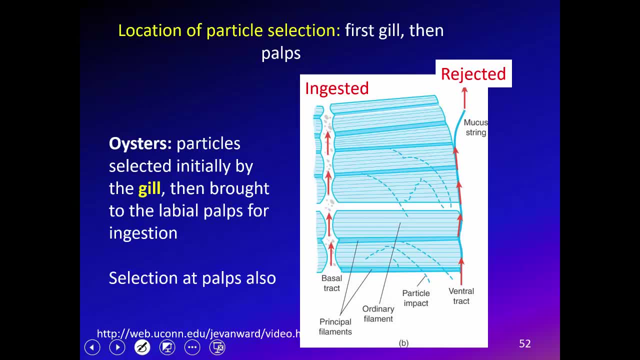 And there is some selection happening before they reach the palps at the gill, And so- and this is what was basically happening- The ventral tract track is where these low particle, low quality particles were being selected for and moved over to the ventral track, in which they, after which they're.